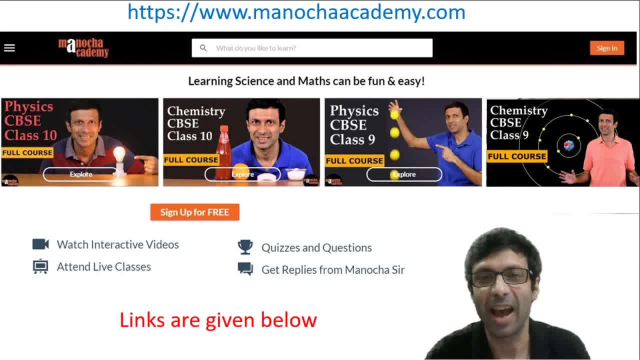 it out. So this is our website, manochacademycom, and I have some great news for you. So just today we've launched the CBSE chemistry class 9 course. So, guys, can you see this course out here? So 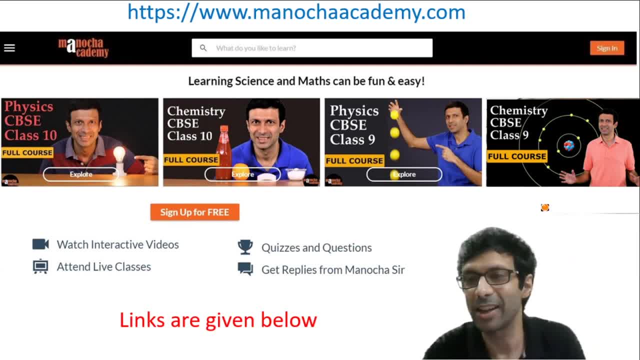 we've launched this course today. So for those of you who are in class 9, we have now the chemistry CBSE course for you, and we also have the physics courses for class 9 and 10 for physics and chemistry, and also the physics CBSE class 9 course. So guys, do check it out. I'll put the links. 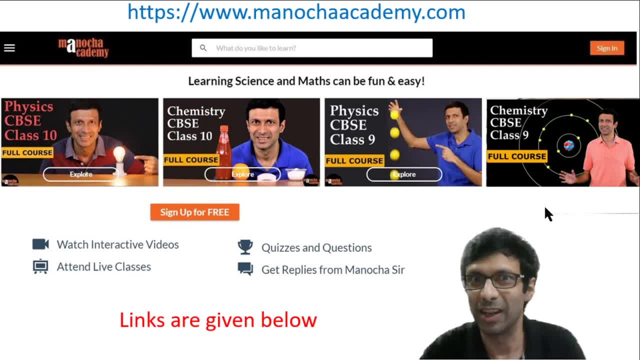 below and we have big discounts going on, So do check it out. So, guys, if you haven't watched our courses, they have interactive videos. You can attend special live classes, There's quizzes and questions and you get direct replies from me. All right, And, guys, if you haven't subscribed to 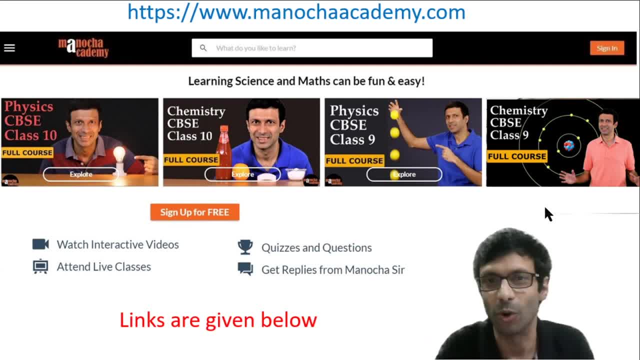 our YouTube channel already. hit the subscribe button right now and click on the notification bell so that you don't miss out on these live classes or new videos that we upload. And guys, be sure to hit the like button for this video and share it out with your friends. So good evening. 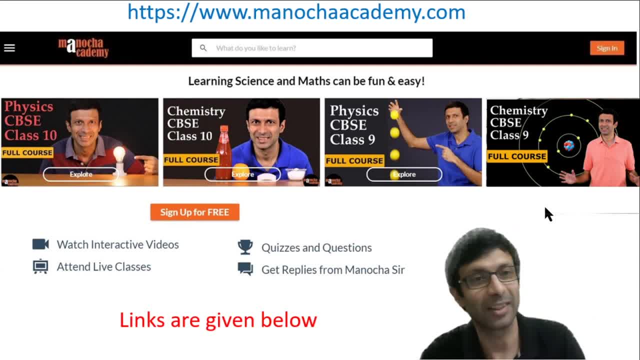 everyone. I see a lot of folks are out here, So, yeah, thanks for subscribing guys, and it's really great to read everyone's comments. So big thanks from the whole Manocha Academy team and please share it out with your friends so that we have. 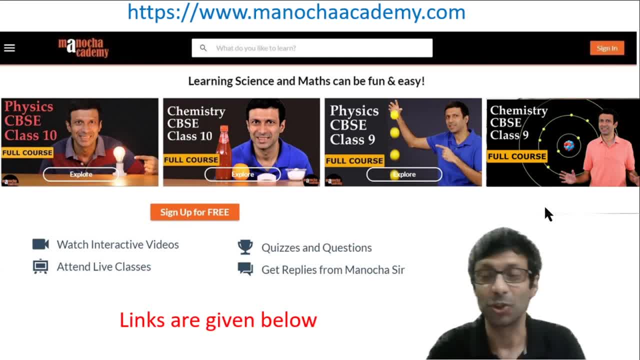 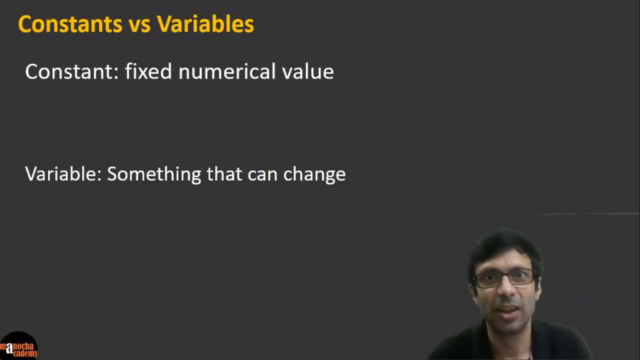 more people on our Manocha Academy family. So, guys, are you excited for this maths class on polynomials? So let's start. So first let's get the basic terms right, right. So what is the constant and what is a variable? 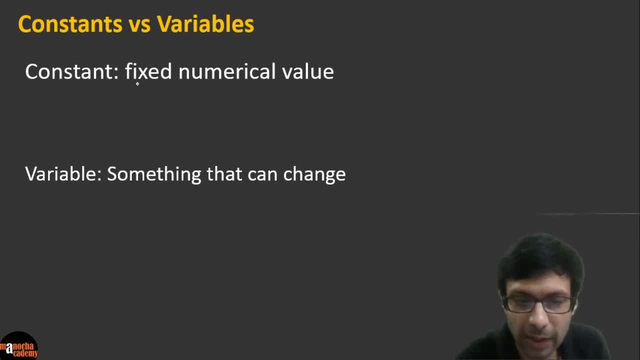 Okay, guys. So what is a constant? So, constant is something which has a fixed numerical value. So can you guys give me some examples of constants? So what are constants, guys? So let's write down some examples here. 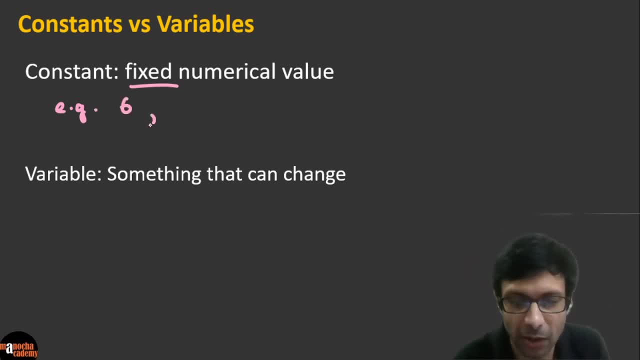 Okay, 6, very good. 6 is a constant. 3, we can say right. 2 or minus 2, right, Very good. So these are all numerical values that are constants, and even a square root of 2, because these values are fixed, They don't change. okay, And what is a variable? 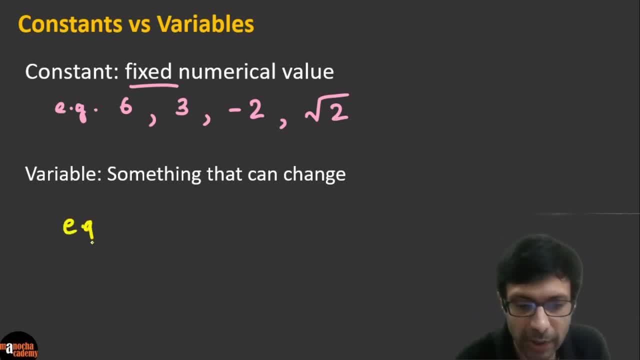 Variable is something that can change. So, for example, we use the notation x right in maths, or y or z, or if you're using the Greek letters right, Alpha, beta. These represent variables which can take different values. okay, So they can take certain. 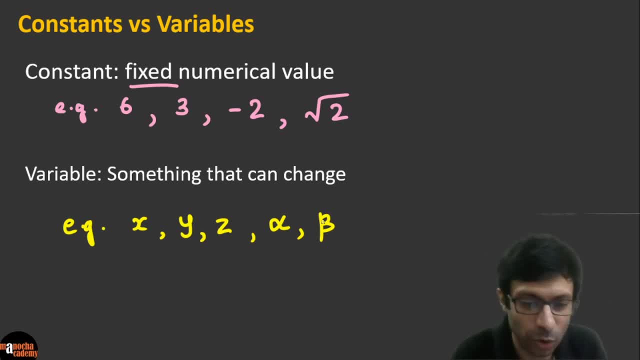 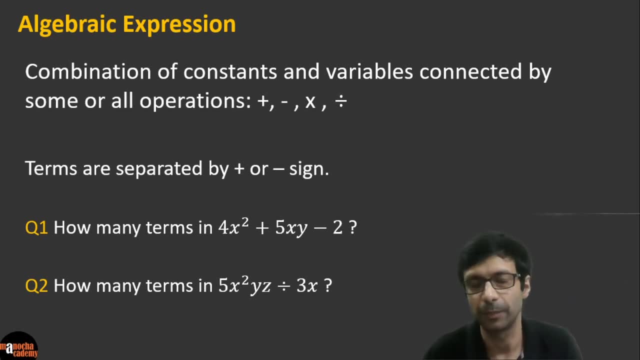 variables. They can change and they can take different values. clear, So this is what is a constant and what is a variable. Now let's be clear What is an algebraic expression, guys? So, combination of constants and variables that are connected by these operations, right So? 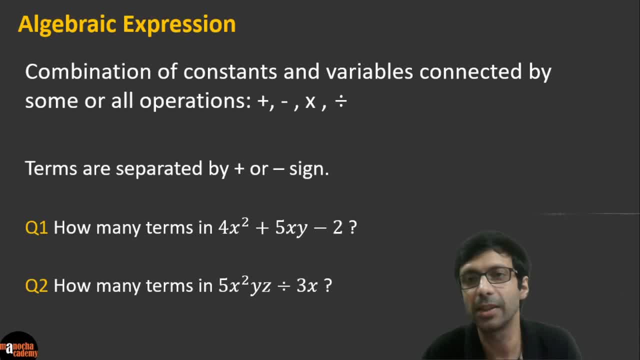 some of these operations or all of them. So plus, minus, multiplication or division, right These operations? So when they're used to connect the constant and variables, we call it an algebraic expression. okay, So you're connecting constant and variables using these operations. 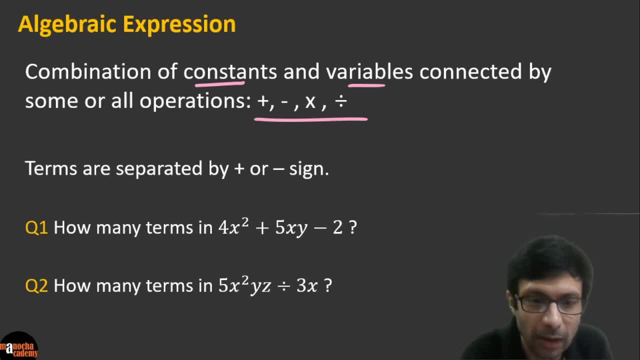 So we say the terms are separated by the, and these terms are separated by a positive or a, so by a plus or a minus, right guys? So now can you tell me the first question: How many terms do you see in this algebraic expression? So here we have an example here for you: 4x squared plus. 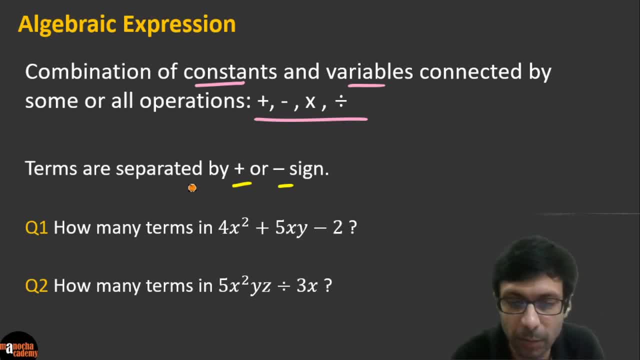 2. So, guys, can you tell me how many terms are there and note that terms are separated by plus or minus. okay, So very good, I see a lot of people are interacting. That's the goal here. I want all of you to try, guys. So go ahead and tell me how many terms do you see here? 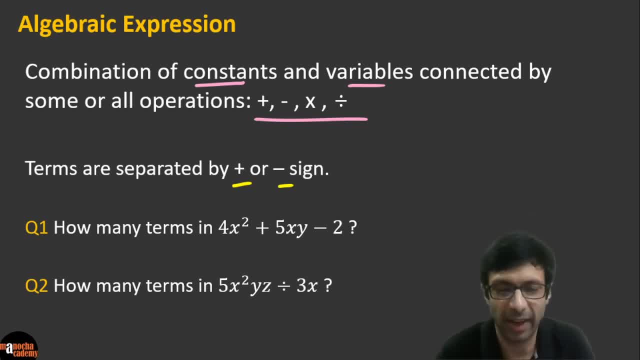 So I want everybody to try guys. Very good, Excellent, I see the right answer here: Superb. So there are three terms in this algebraic expression, right? Can you see the three terms here? 4x squared plus 2.. So there are three terms in this algebraic expression, right? 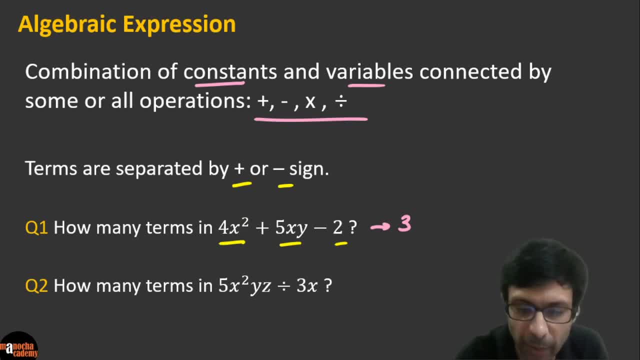 5xy and 2, because they are separated by this plus. can you see the plus here? so they're separated by the plus and the minus. okay, excellent guys. so now in the second question, can you tell me how many terms are there in 5x squared yz. 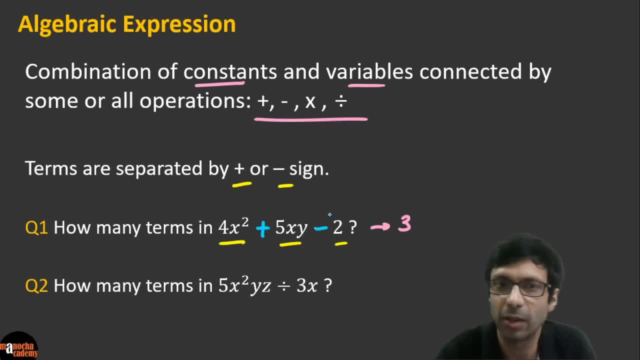 divided by 3x. so how many terms guys do you see in this? okay, so some of you are saying one, some of you are saying two. okay, one term, two terms. guys decide. what do you think is the answer here? so note that. what is the key point? that terms. 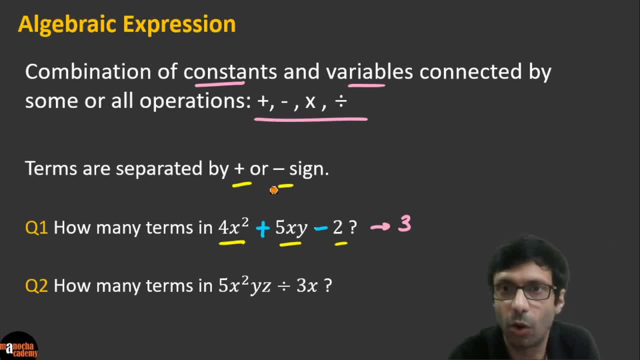 have to be separated by a, only by a plus or a minus. right, so everything can be combined using plus, minus, multiplication or division, but for each term it is only separated by a plus or a minus. and here, guys, you can see that there is no plus or minus, we just have a. 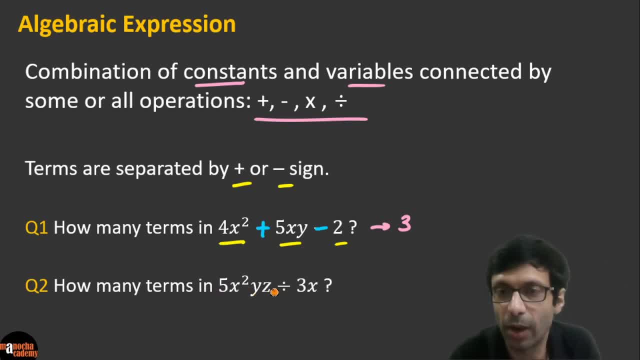 plus or minus. we just have a plus or minus, we just have a division here. and of course these are x square by z. these are all multiplied within right. so we just have a division here. so that's right. very good, a lot of you have got the correct answer. there's only one term here, because there's no. 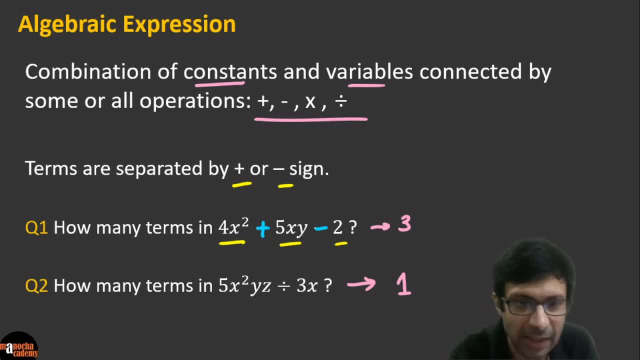 plus minus. so it's just a division and this entire thing is just a single term. so this is one term, very good guys. and so when we write an algebraic expression, for example, if you see this, we say that this is the first term. right, this is the second term and this is the third. third. 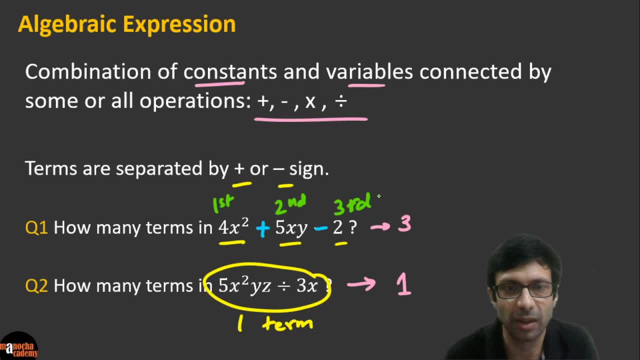 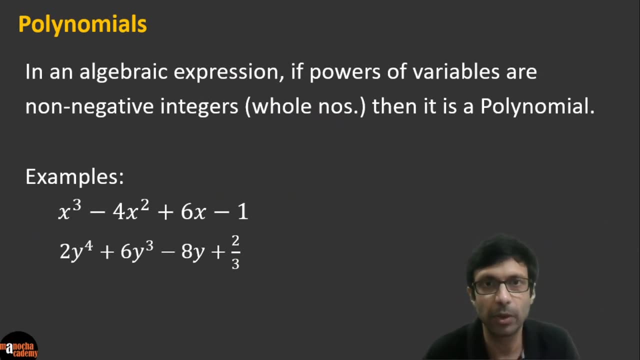 term right, so we can give the terms certain numbers. okay, very good, so you got the concept here. don't confuse with all the operations. the terms are separated only by a plus or a minus. great, now let's see. so we talked about constant and variables and algebraic expressions. now let's learn what is the polynomial. 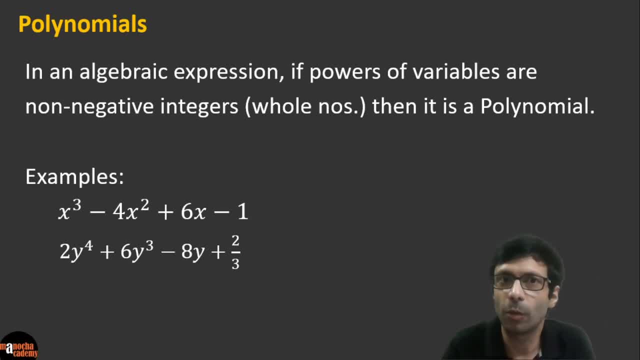 which is the topic for today's class, right? so let's learn what is the polynomial, which is the topic for today's class, right? so polynomial if in an algebraic expression, if powers of variables are non-negative integers, okay. so when you take an algebraic expression, if the 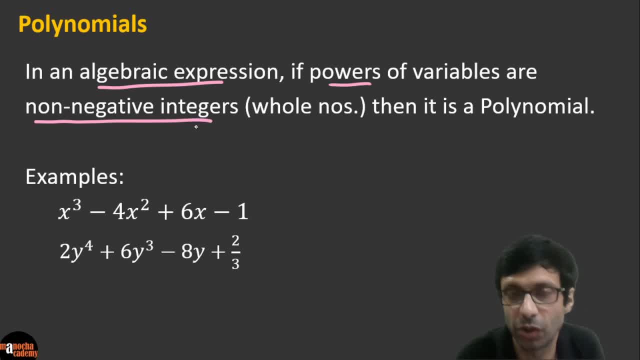 powers are non negative integers, which in other words, you know we can say they are whole numbers, right? so what are non negative integers? so you can have zero, one, two, three and so on. so if the powers of the variables are these, then it is a polynomial, polynomial, right. so let's take a look at some examples here. so, guys, take a look at the first. 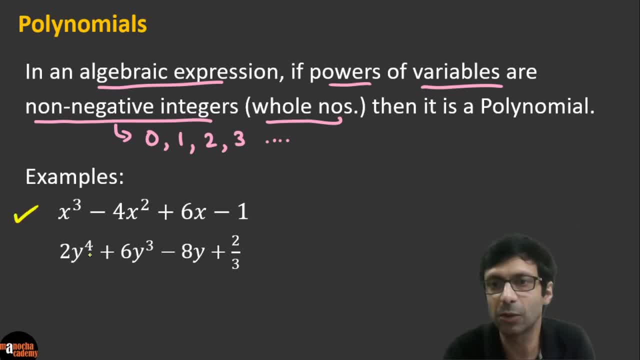 example: x cube minus 4x square plus 6x minus 1. okay, so what is the variable here? here you can see: the variable is x, right? x is our variable. and now follow the powers here. so it's x to the power. 3, right, so that's a whole number. then you have x square here and x is basically x to the power. 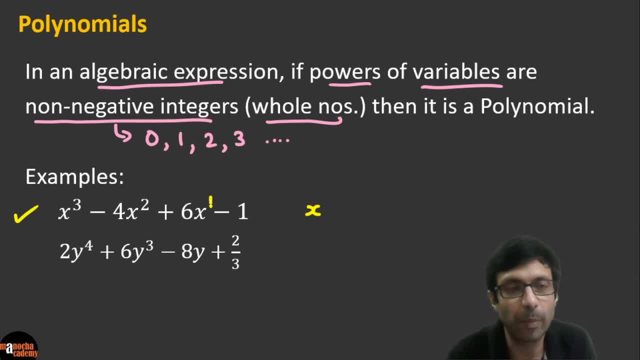 1, right. so can you see that all the powers are whole numbers. so this is a, definitely a polynomial. that's why it's an example of a polynomial in x. right and guys. so this is a polynomial in x. and look at the next one. so is the second example also a polynomial? 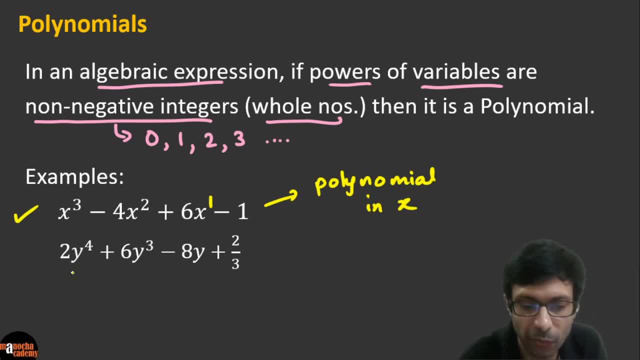 right, because, can you see here, the variable is y here and you can see that all the powers y to the power 4, y cube, and you have y which is y to the power 1. so these are all non-negative integers and we don't care. 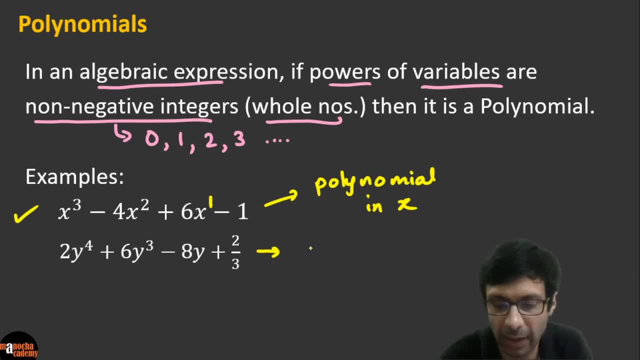 about 2 by 3, because there's no power of y right in that case. so this, this is a polynomial in y, the second one right, clear guys. so get your concepts clear so that you're not confused by these terms, because a lot of these are asked in the multiple choice questions where you really 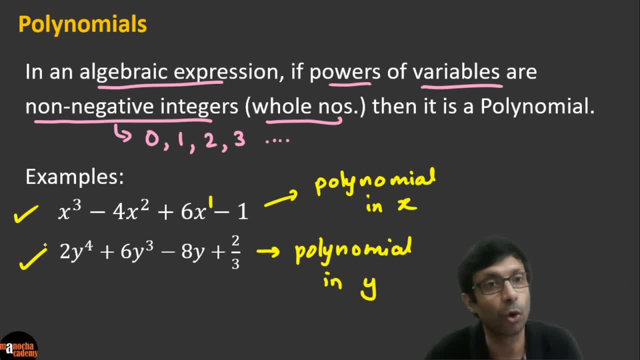 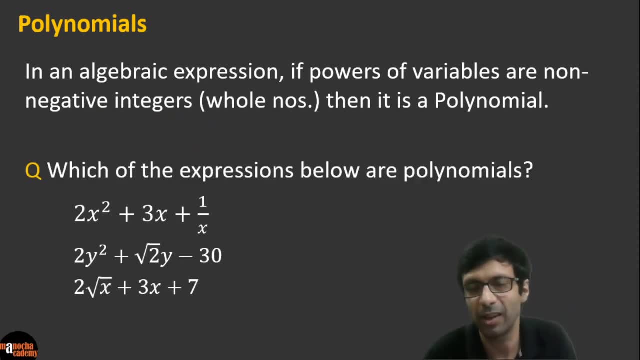 need to understand the terms in the chapter, these basics, before you proceed to the chapter, and that's going to be the focus of the class: to really understand polynomials completely right and be crystal clear about it. so this was our definition, and now i have this question for you. 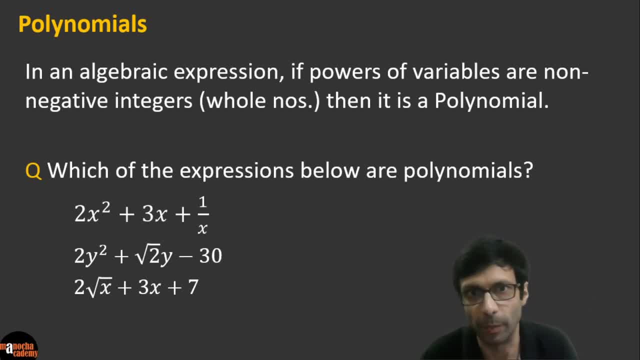 which of the expression below are polynomials? right, so can you find the polynomials here and let me number them for you. so this is number 1, 2 and 3. so, guys, take a look at your screen and tell me which of the expressions below are polynomials and which of the expressions below are polynomials. 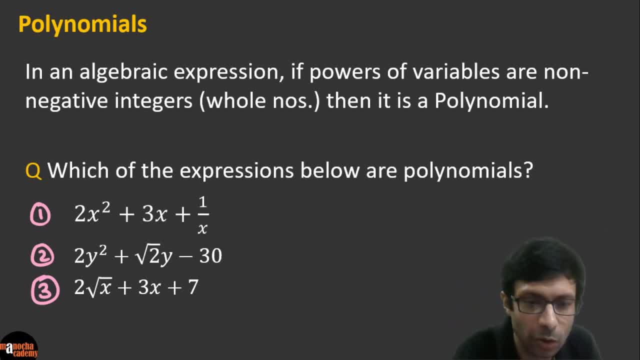 and i have the definition up here for you so all of you can see the definition here, right? so take a careful look and tell me what do you guys think are polynomials? okay, so some people are saying two, one and three. okay, some are saying three. so take a careful look, guys. remember the. 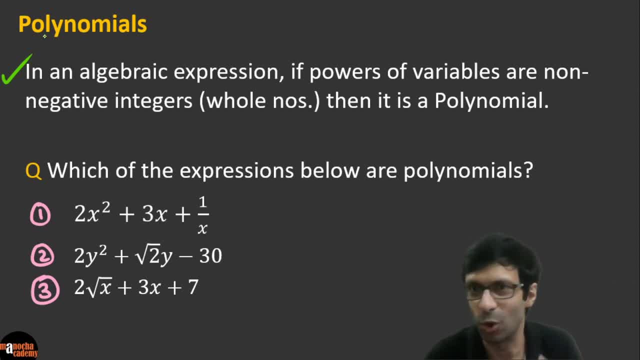 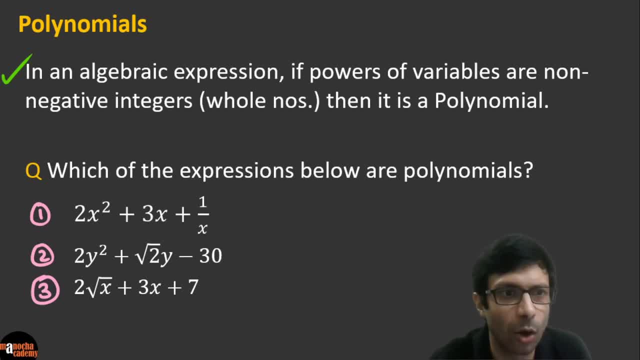 and i'm looking at the chart here, guys. so come on, uh, all of you try, and, guys, if you haven't hit the like button for this class, please hit the like button right now, uh, and do share it with your friends. so take a look at my question, and which one do you think of these expressions? so, 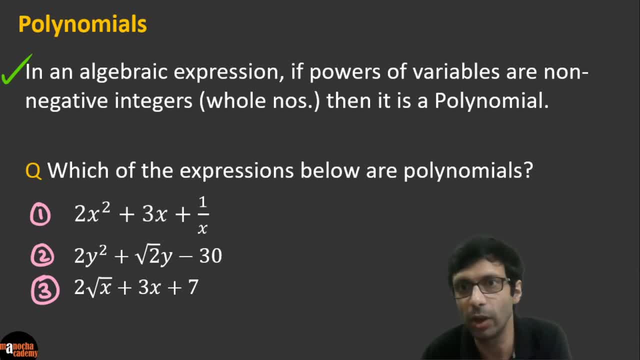 we call them algebraic expressions and they are polynomials- only if it satisfies the above definition there. okay, so let's go one by one and you guys check your answer. i see a lot of answers here. it's really great to see that, uh, so let's uh go ahead and look at the first one here, right? 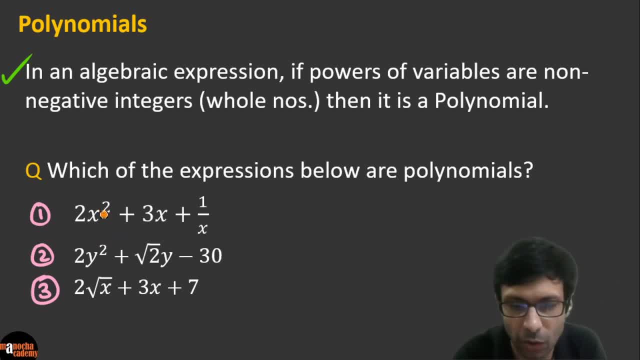 so first one. you can see it's x squared, so that's a whole number. this is x to the power one. but if you look at this term, 1 by x is basically the last term is x to the power minus 1 right. 1 by x is: 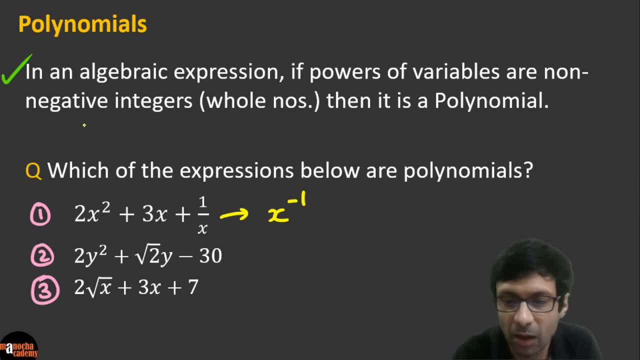 nothing but x to the power minus 1, and that is a negative integer. so the first one is not a polynomial, it's just an algebraic expression. okay, guys, now go to the next one. right? so do you guys agree with me? because there's x to the power minus 1, negative part, it's not a polynomial. 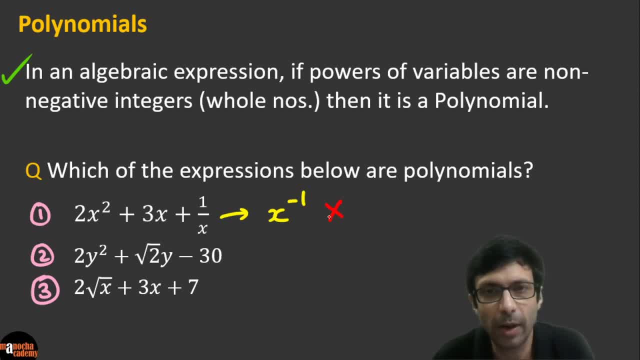 right now. let's take a look at the next one: 2y squared plus root, 2y minus 30.. so if you look at the first term, it's y squared, so that's okay. 2. this is y, or basically y to the power, 1 right and minus 30. there's no power of y, so we don't look at that. 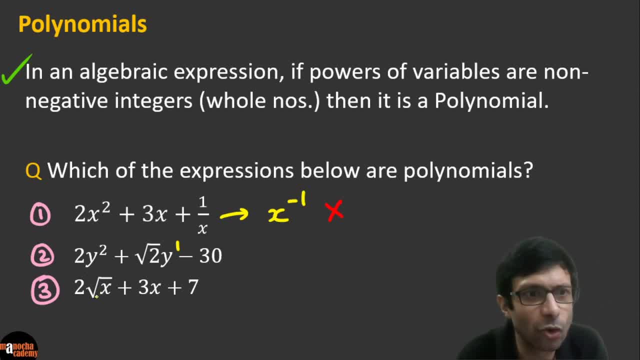 so can you see the second one, guys, very good. i see dhruv gupta says 2 is uh, right, right, okay, so great, so this one is correct, very good. uh, srinivas also says that so 2 is definitely a polynomial because non-negative integer. and, guys, now you uh take a look at 3 and tell me, is 3 also? 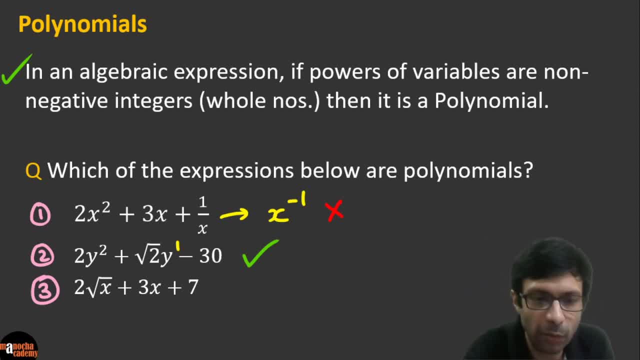 a polynomial, okay. so if you look at 3 carefully, what do we see here? it's basically so. this is. uh, the first term is 2 root x. so root x we can write as 2 into x to the power half. right, guys, you know this, that root x means x to the power half. 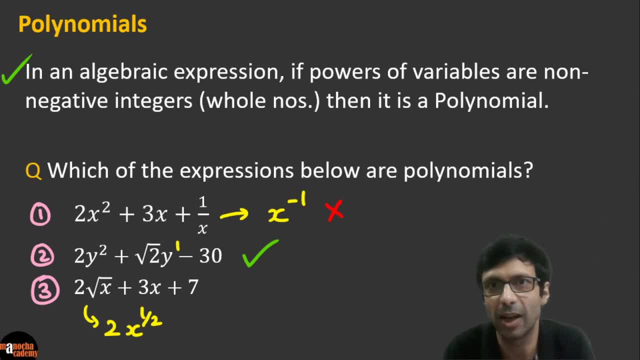 okay, and there you can see that a fraction has come. it's not an integer power, so therefore this one is not a polynomial. so very good, those of you got it. the only polynomial here is number two. okay, clear guys. excellent, let's move on. so is everyone clear about that? all right? 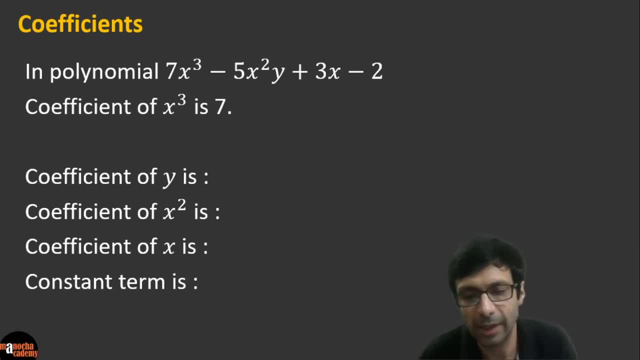 now let's talk about the coefficients in the polynomial. so if you take a look at this polynomial, i have given there right and this polynomial contains both variables x and y, as you can see. so it's 7x cube minus 5x squared, plus 3x minus 2.. so in this you can see, here's an. 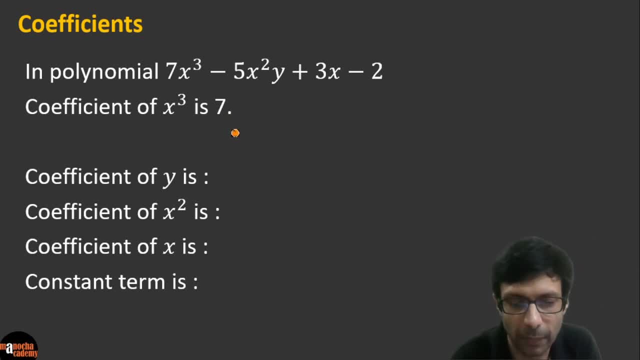 example, the coefficient of x cube is 7, right? so coefficient of x cube means so if you look at xq, the part that's remaining in the term right, can you see 7. so we say 7 is the coefficient of x cube. so, guys, can you tell me what is the coefficient of? 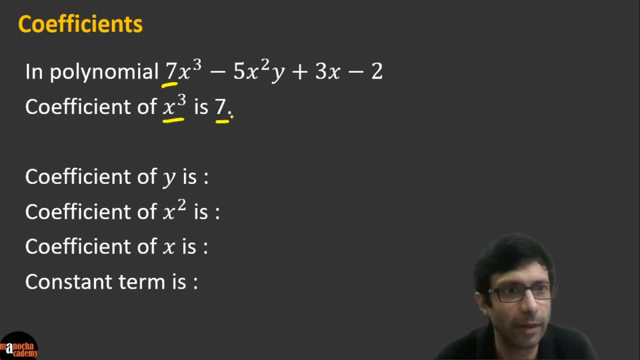 y in that polynomial, okay. so who can tell me what is the coefficient of y? and hint is, it is the part remaining, the remaining part in the term, okay. so all of you try. some of you are saying 5x squared, some are saying 5, okay. so see this confusion and i want all of you guys to be crystal clear, right. 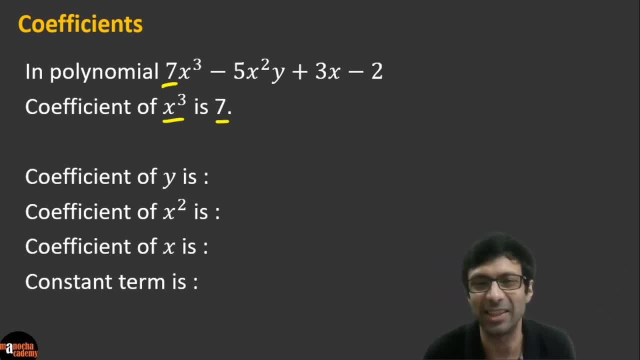 these terms so that you find max absolutely easy. so, guys, come on, try, try out this. so what is coefficient of y? so how will you solve this? very simple, so if you take a look at y here, so this is y and what is the remaining part? so let's mark the remaining part here. 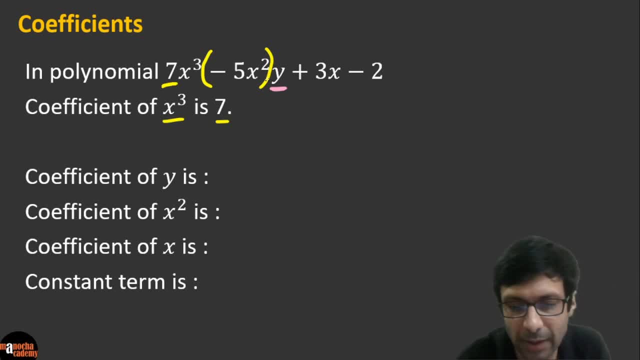 so the remaining part is not just 5x squared, but the minus sign also. okay, so don't forget to take the negative sign. that's a common mistake. so the coefficient of y is minus 5x. okay, we don't write if it's positive. we don't write plus 7, right, but the negative sign has to. 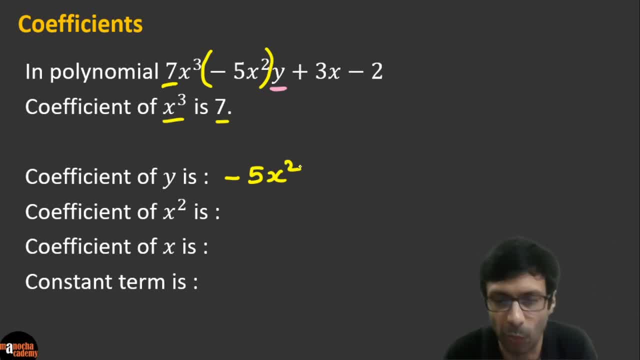 be written: okay, so minus 5, the part remaining from y. very good, and let's take a look at what is the coefficient of x here, or, sorry, what is the coefficient of x squared? the next one, okay, so if you look at again at this term, right, so the term here was given as minus 5x squared y. 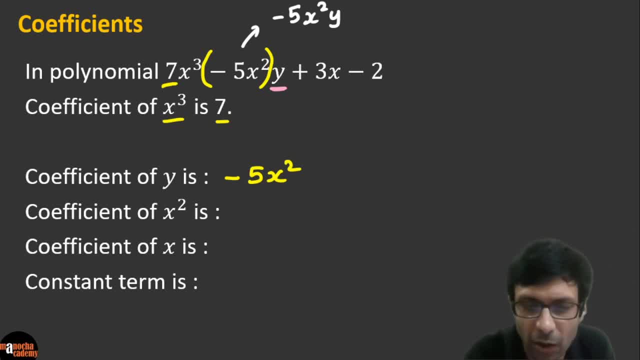 the second term, and there are some other terms that are given as minus 5x squared- y, the second term- and they are asking what is the coefficient of x squared? so we'll look at that and see what is the remaining part. and the remaining part, guys, you can see simple, it's minus 5 y, right? so the part that 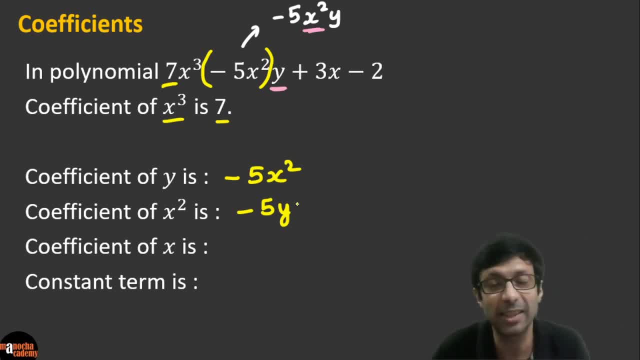 remains very good. i see a lot of you written minus 5 y and note: guys, it's not minus 5, you have to include the y. so in that term, whatever is remaining clear, okay now, what is the coefficient of x here in this polynomial right? so, guys, 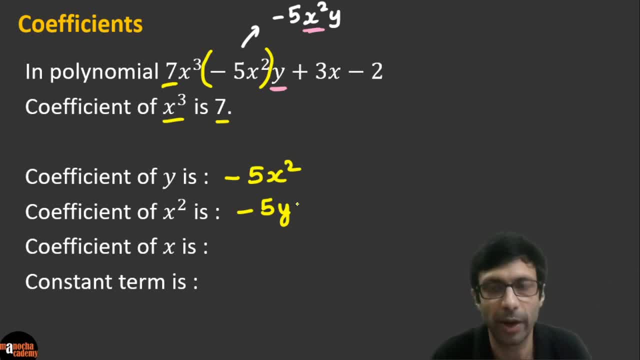 what is the coefficient of x? okay, very good. so some of you have written the answer, the part which remains, and that's 3. great, and the constant term: right. so the constant term, remember, there's no variable here, it's a fixed value. the constant term is again, not 2, it's going to be minus 2. 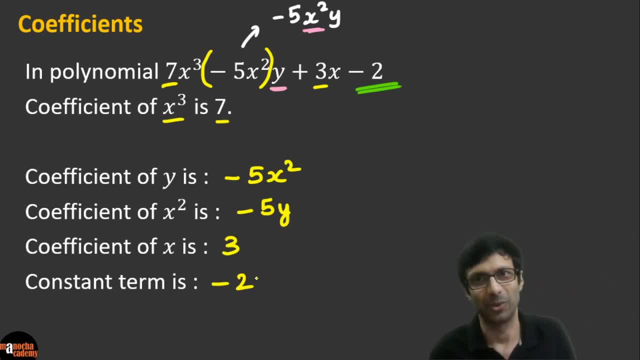 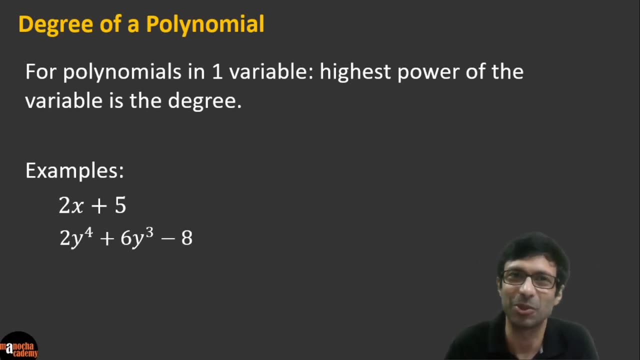 so what is the moral of the story? don't forget the sign, okay, because in these coefficients you have to include the negative sign, if it's there. so, guys, it's not 2, it's minus 2. clear, excellent. now let's talk about okay. this chapter is full of so many terms, right? so 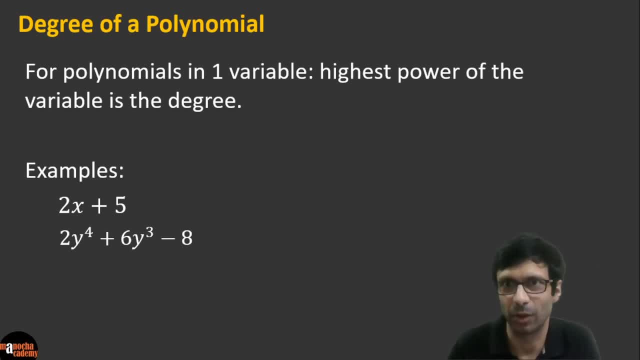 now let's talk about what is the degree of a polynomial. okay, so for polynomials in one variable, that means if it's just x in the polynomial or just y, the highest power of the variable is the degree, right? so the highest power that the variable takes in the polynomial? 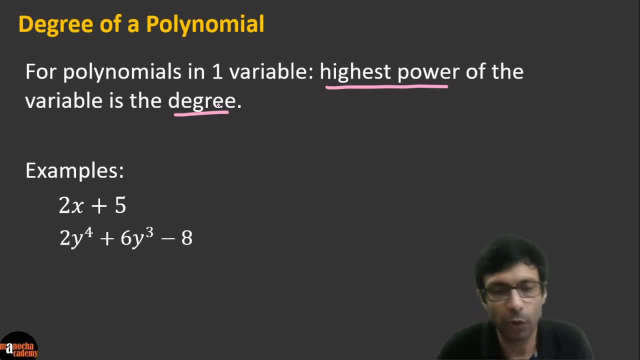 degree. okay. so, guys, can you tell me for the first polynomial here, so for 2x plus 5, what is the degree? so we are writing down the degree of these polynomials. so who can tell me what is the degree of the first one? wow, you guys already have the answer. you guys rock very good because you can. 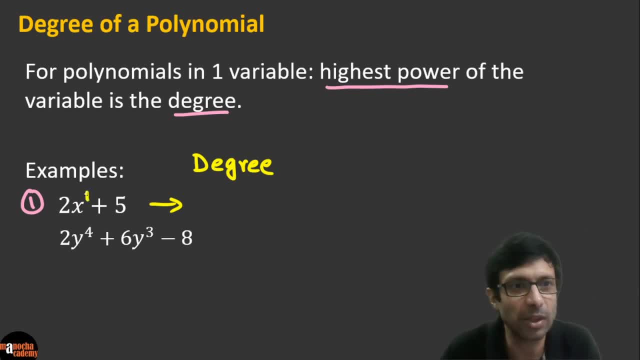 see it's 2 into x, 2 times x to the power 1. okay, so fantastic guys. so it's simple here. degree is 1.. so that's right. get your concepts and definitions clear, then all these questions will seem really easy to you and guys, can you tell me what is for the second one? what is the degree of the? 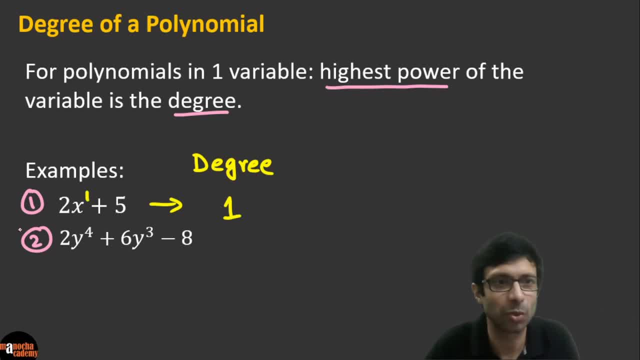 polynomial. and note this: polynomial is in y, it can be in x, y, whatever variable. so, guys, what is it? excellent, excellent. i see the right answer here. the answer is 4.. clear. so degree is the highest power of the variable. can you see the highest power? here y to the power, 4, and here the highest. 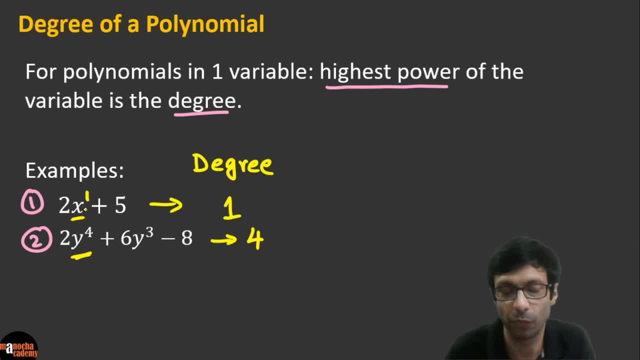 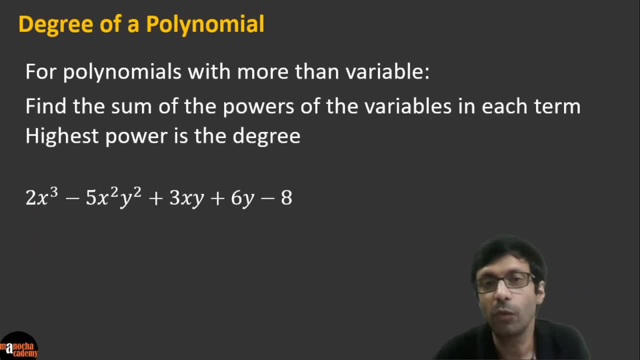 power is x to the power 1, right, don't forget, it's x to the power 1, not just x, right? so great now if you have polynomials with more than one variable. so sometimes you might see this in your books, right? so can you see this example over here? it is a polynomial in x. 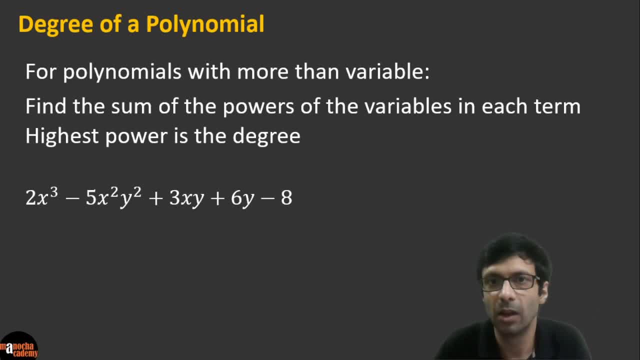 and y, so not just one variable. there are two variables here. so how do you define the degree of that? so what is the technique? let me show you. you need to. the definition is: you need to find the sum of the powers of the variables in each term right, and then the highest power. 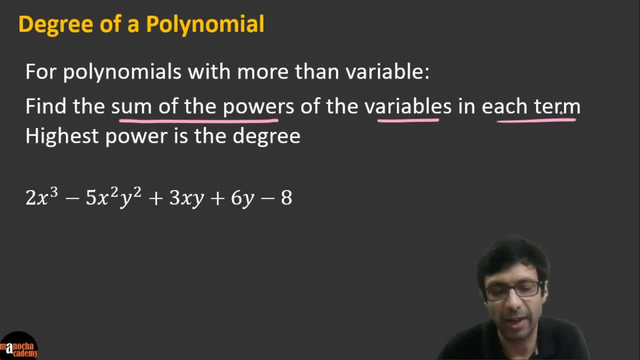 is going to be the degree, okay, so, guys, let's do this one together. so take a look at this polynomial and we need to find its degree and note. the interesting thing is it's a polynomial in two variables. right, it's a polynomial in x and y- clear, 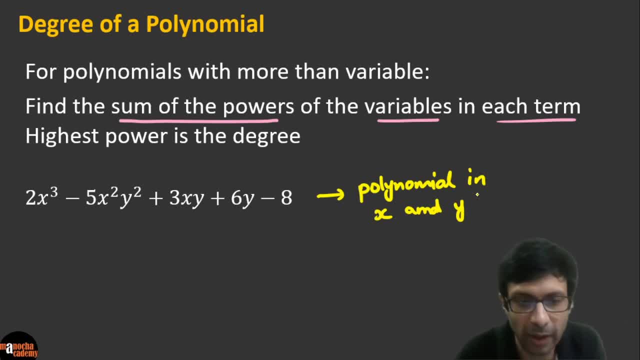 okay. so let's look at our first term here. so 2x cube, right, so we need to find the sum of the powers of variables in each term. so here there's only the variable x, right, so we can write what is the degree of this term. right, so we can say the degree here is 3, right, okay, because it's. 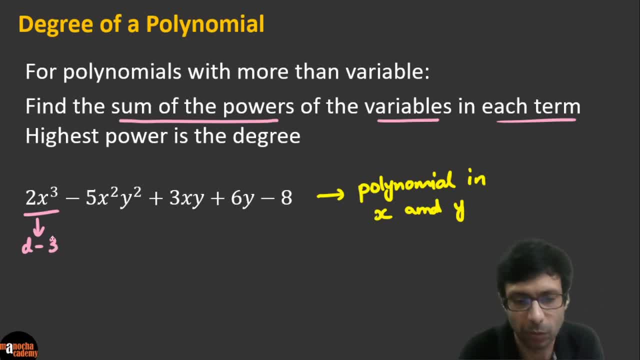 right x to the power 3.. so we can write the degree of this term right. so we can say the degree here is 3.. now take a look at this term. so if we just look at this, what would the degree be of this term? right 2 plus 2, because it's x squared and y squared, so we need to add the powers, so we 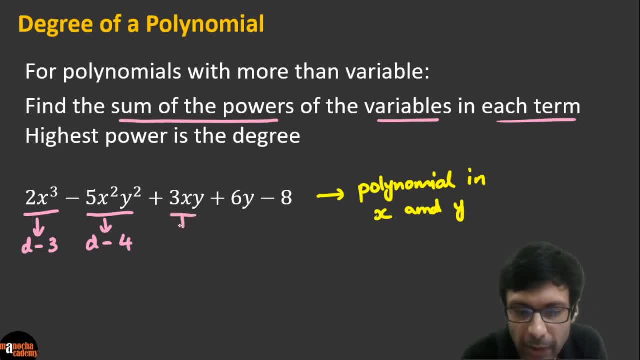 need to add 2 plus 2, so that's 4.. so you can write it clearly like this, so you have no confusion. then 3 x, y, it's going to be degree 2 if you look at this term, and this one is going to be. 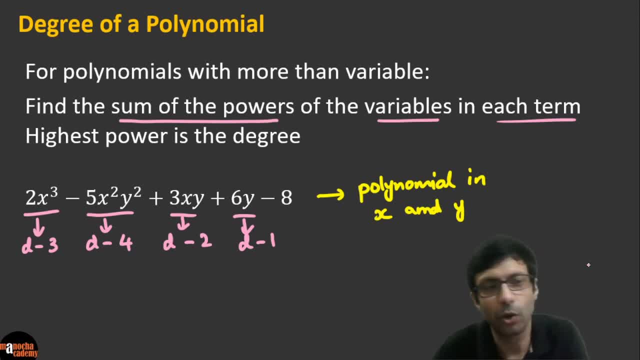 degree 1. right, because it's y to the power 1.. very good, i see a lot of you have the right answer. so what is the highest power? out of all the terms and guys, you can see that the highest power is 4. right, because in that second term, can you see, it's x squared by. 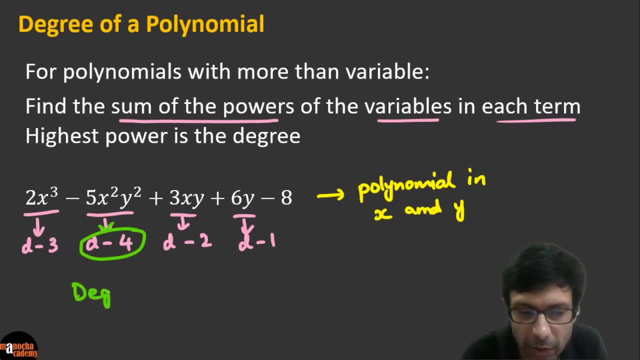 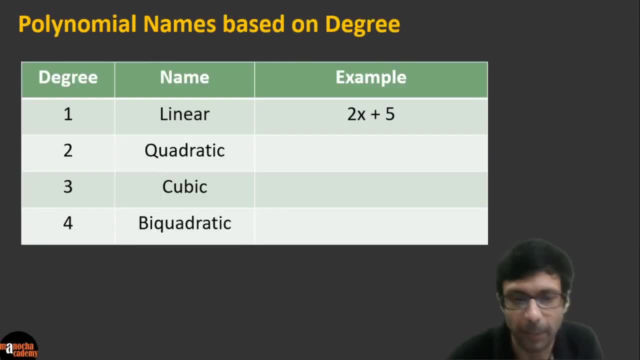 squared, so 2 plus 2. therefore, the degree of this polynomial is going to be 4.. clear, very good, excellent. all of you got that very good. so now we can give the polynomials names based on the degree, the highest part that we talked about, right? so i have an example. 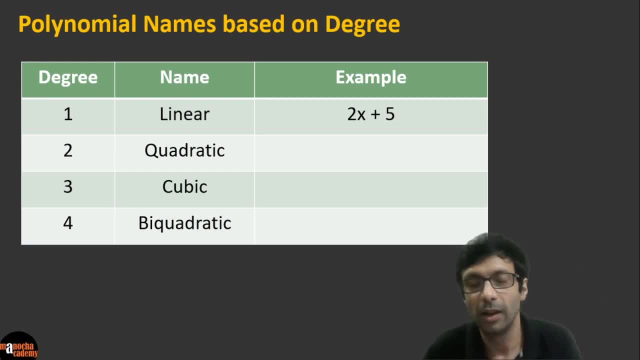 here for you. so if we say we're looking at a degree 1 polynomial, it's called a linear polynomial. and here's an example: 2x plus 5, right? if you're looking at a degree 2 polynomial, right? so let's take an example. let's say the polynomial is x squared plus 3x. 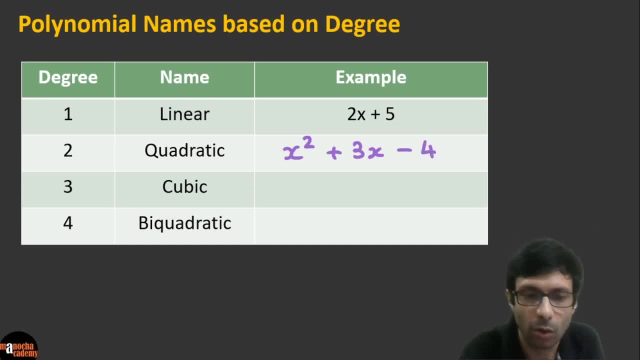 minus 4. okay, so this is called a quadratic polynomial. do you see that it's a quadratic polynomial? because it's, uh, the degree is 2. here the highest power is 2.. when the degree is 3, it's called a cubic polynomial. so an example would be something like 2x cube right minus 5x squared. 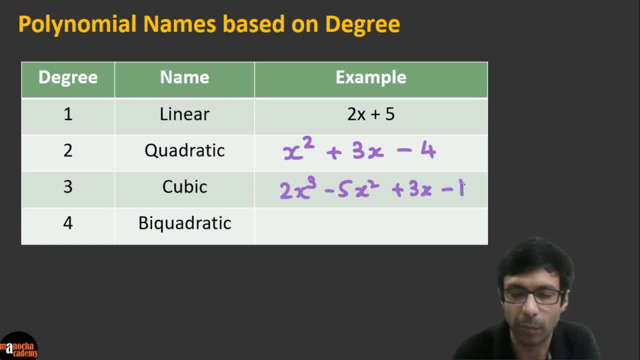 plus 3x minus 1 right, whatever example. but here you can see, the highest power is 3.. so it's uh, degree 3, it's called cubic, and similarly, if the degree is 4, it's called biquantratic. okay, so let me write an example. let's say x to the power, 4 plus x cube right minus 3x squared. 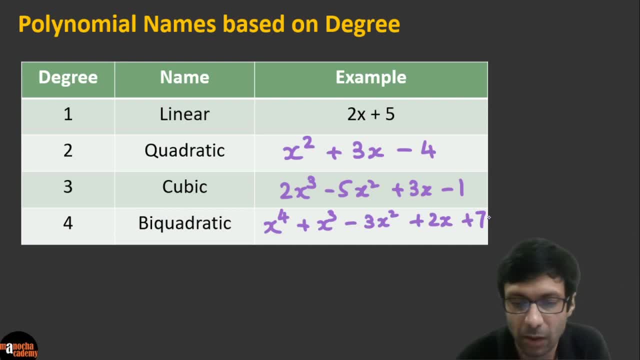 plus 2x plus 7, so this is a biquadratic polynomial. clear, because the degree is 4.. so you need to learn these terms and names so that you won't get confused. so there are a lot of terms in this chapter. right and uh? so these were the names of the polynomial based on degree. now you can give. 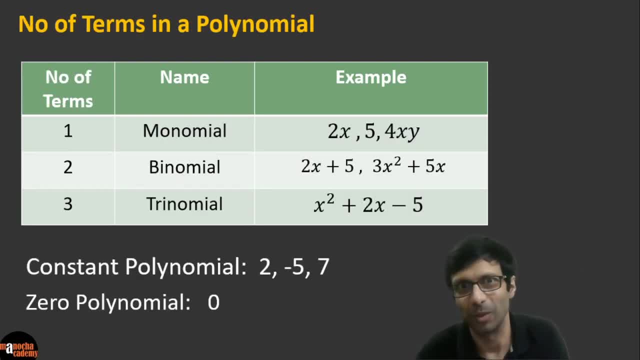 the names based on the number of terms, also in the polynomial, okay. so, guys, if you look at, if a polynomial has one terms- remember we talked about the terms are separated by plus or minus, right by an addition or subtraction, so by plus, minus if it has only one term, like for. 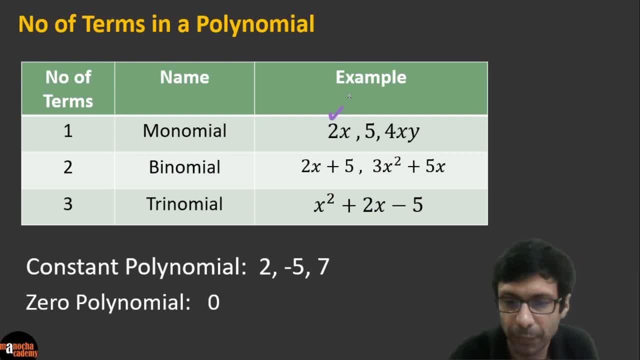 example, if you have these polynomials right, let's say a 2x or a 5 right, the constant term or 4xy right, these are all known as mono monomials right. mono means one right, so these are called monomial right. and now if it has two terms, like if you take a look here: 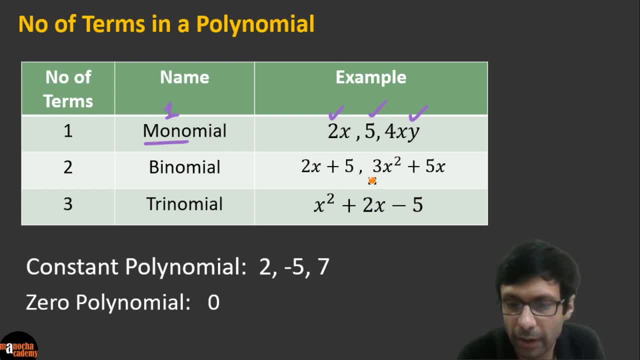 2x plus 5, right, or can you see there are two terms: 2x and 5. then, if you look at this example, 3x squared and 5x, so there are two terms here. this is called a binomial by means two. 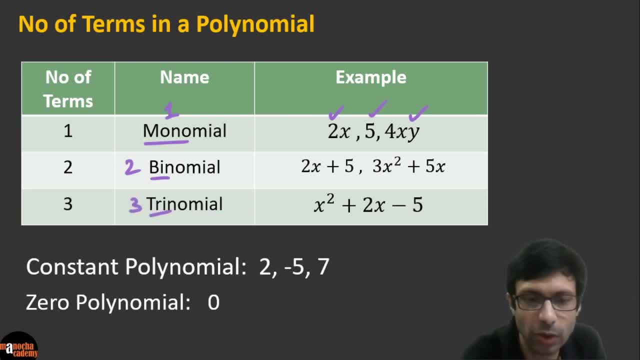 right, and similarly you can see trinomial. can you see that, guys? it has three terms here. okay, now there are some more terms of things. in polynomials you have something called a constant polynomial, so something which just has a constant right. so even two is considered a polynomial. but 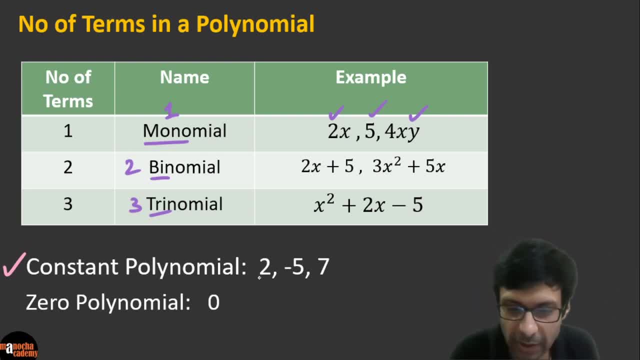 it's called a constant polynomial because there's no variables there. so these are some examples for you. so here i've written down these examples. right? so 2 is a constant polynomial, or minus 5 or 7, right? these are examples of constant polynomial and zero polynomial, a very special one. 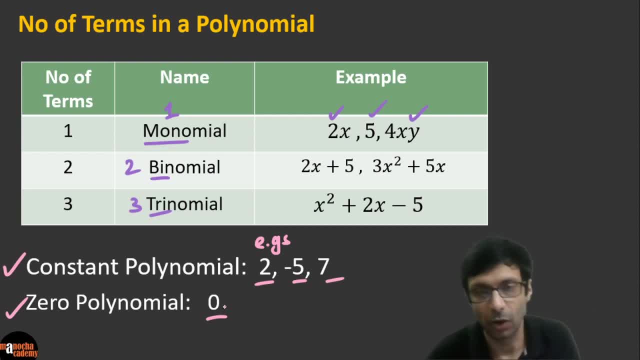 is just a number zero, right, okay. so now can you tell me an interesting question. let me ask you: what is going to be the degree? so what is the degree of constant polynomials? so these guys, so who can tell me what is the degree of the constant polynomial? so let's say you take the 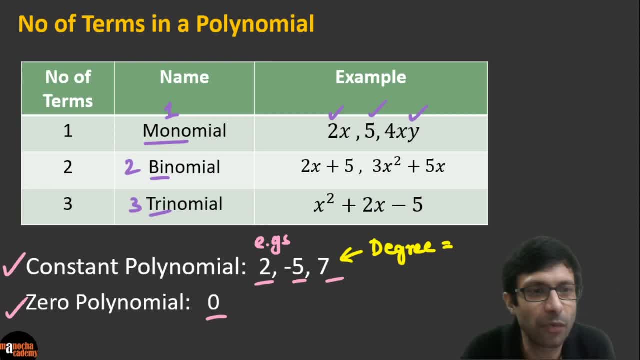 example 2. what is the degree? okay, very good, excellent. i'm seeing a lot of answers here, some of you saying zero, some of your say 0, do not know, you're seeing one, so guys decide. so my question is: what is the degree of a constant polynomial? and let's take the example. let's say 2 is a constant. 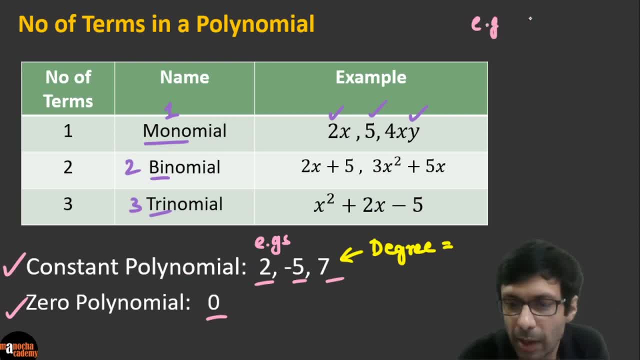 polynomial, right? so let me write it here. so, for example, the number 2, that's considered a constant polynomial because it's just constant, right? very good, so a lot of you got the right answer. the answer is: the degree is going to be 0. right, the degree is 0 because you can think 2 is basically 2 times, if you. 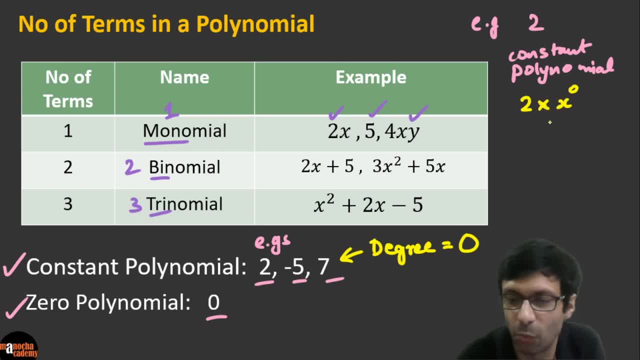 think it this way: X to the power 0 right. X to the power 0 is 1 right, so that's going to be 2 into 1, right. and so the power of the variable is 0 because X is not there, so it's X to the power 0. so the you can know that, you can learn that. 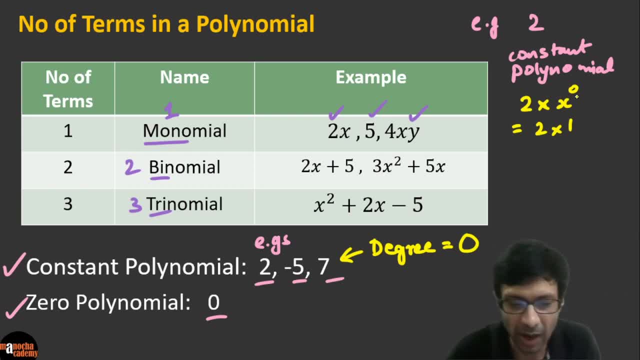 constant polynomials have degree 0. very good. and guys, what is the degree of the 0 polynomial? who can tell me that? 0? So what should I write as the degree of the zero polynomial? okay, So zero polynomial is a special one, and what do you think its degree is? 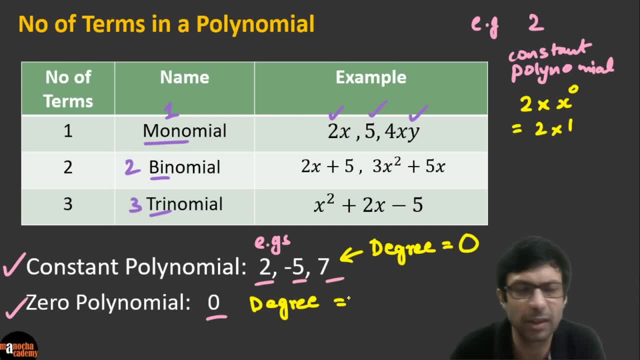 So some of you are saying 0,. some of you are saying 1,. okay, It is great to see all of you trying that right. So let me give you a hint, right? So 0, I can say. so if you take this number, 0,. 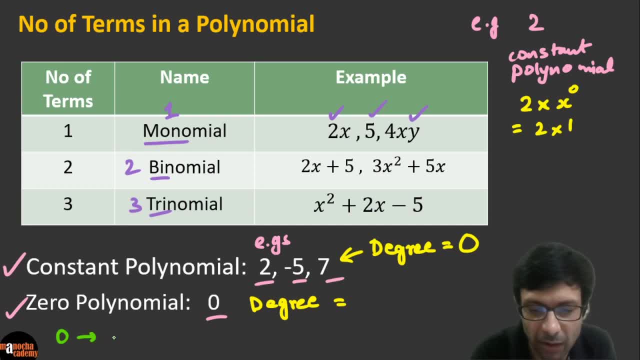 so I can say this: 0 can be 0 times x square, so dot means multiply, right? So 0 times x square, or it could be 0 times x cube, or it could be 0 times x to the power 1, right. 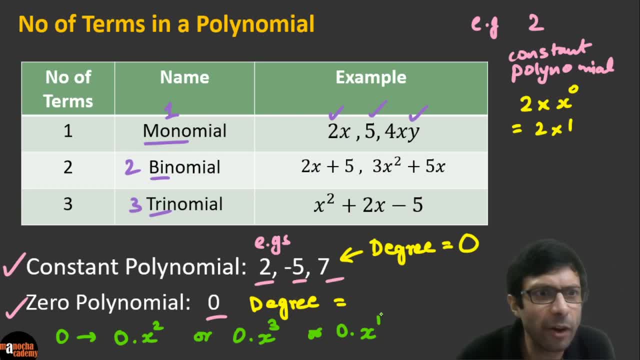 So what do you think is going to be the degree here? right, Very good, I see, Mamta. right, Manjeeta, they have got the right answer. So some of you are saying Infinity? no guys, it is not defined, right. 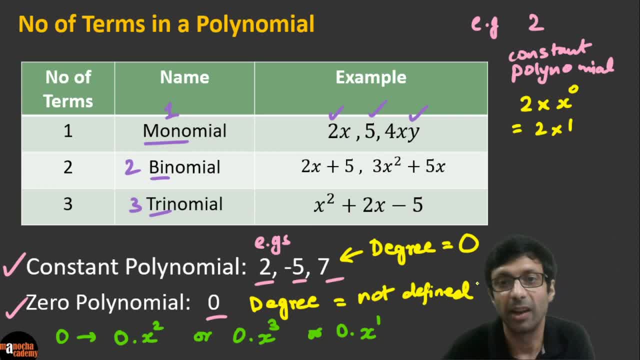 Because it could be anything. As you can see from my examples, it can be 0 times x square, or 0 times x cube, or 0 times, I do not know, x to the power 7.. So the power of x is the degree. 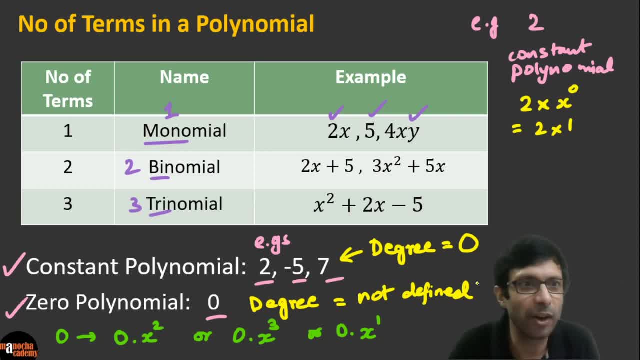 Remember the power of x is not defined here, right? So very good and sorry if I missed your name. Some of you did give the right answer. You know the chat scrolls really fast, So excellent guys, Remember this very tricky question. 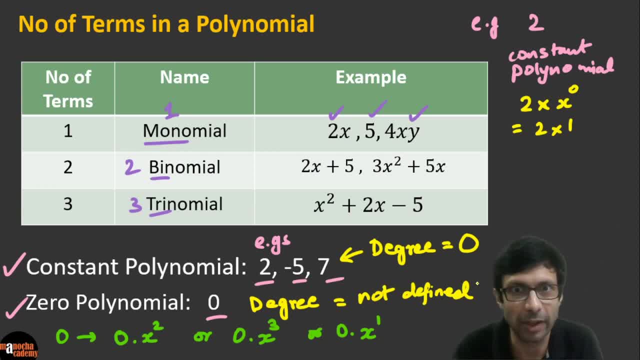 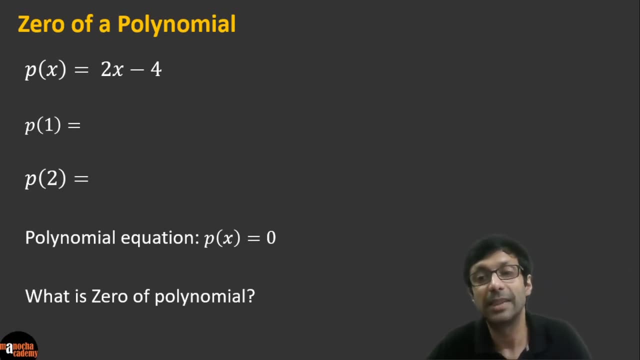 It can come in the MCQs: Constant polynomial. they have degree 0 and I showed you a simple example. But the 0 polynomial, the special guy, is not defined, The degree is not defined- Fantastic guys, Okay. so now let us talk about what is the 0 of a polynomial right? 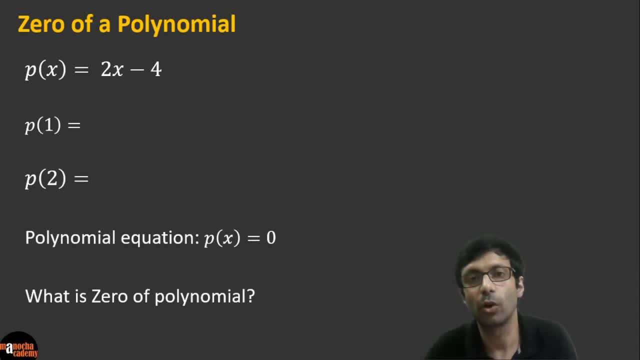 We are not talking about 0 polynomial. That is done right. So now we are going to talk what is the 0 of a polynomial. So let us discuss that. So before we talk about that, let us take this polynomial here. 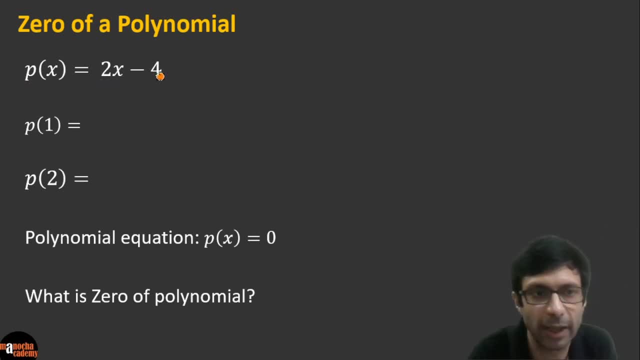 Let us take a simple polynomial, px as 2x minus 4, okay, So how do we find p of 1?? So what is p of 1?? Very simple, You just have to take the polynomial. So we just need to substitute x equal to 1 in this polynomial. that is all right. 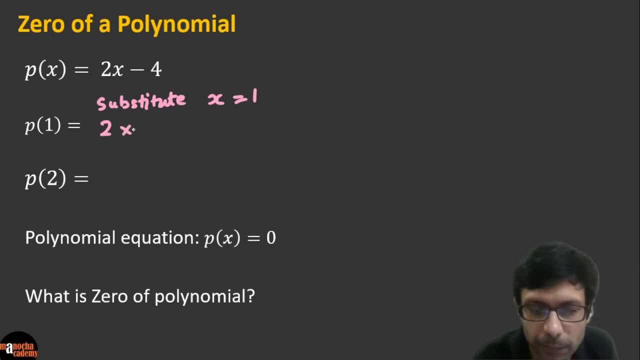 So it is going to be 2 times 1.. Right Minus 4.. So what is p of 1? going to be Very good, You guys got it right. So we are just substituting the value. 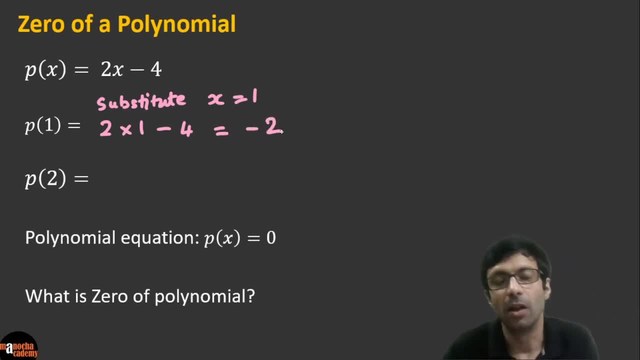 So 2 minus 4 is minus 2.. Simple. Now, what is going to be? p of 2, right? So if you look at the notation, basically the number that is given in the brackets, right, We are just substituting, because x is taking this value- the variable x. 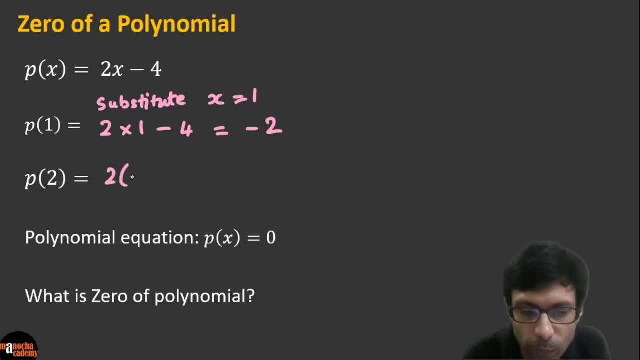 So again, we just have to substitute: So 2 times 2,, right? Okay, So it's going to be 2 times 2 minus 4, and what do we get? 0. So basically, we've got here that p of. 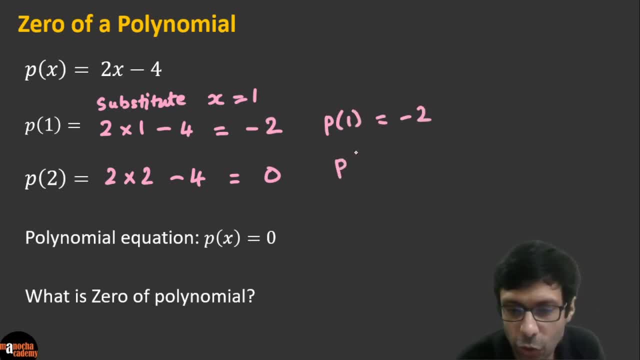 1 is minus 2, p of 2 is 0, and similarly we can find p of 3, p of minus 1, minus 2, right? So we can find these values right. So what is the basic trick? You just substitute it into the polynomial. 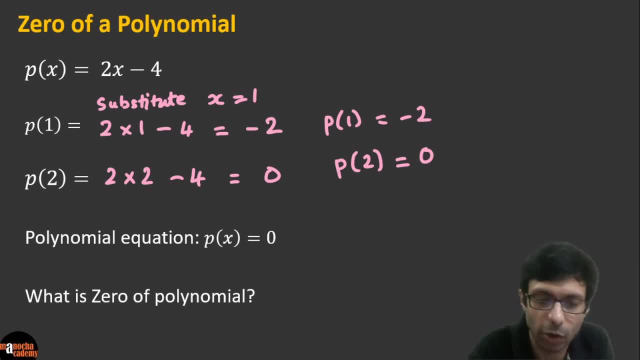 okay. So now, if we take this polynomial px right, or any polynomial, if we take px and we equate it to be 0.. So guys carefully follow me here. So if we take the polynomial px right and we say: set that equal to 0, we are basically forming a polynomial equation, right, Can you see? 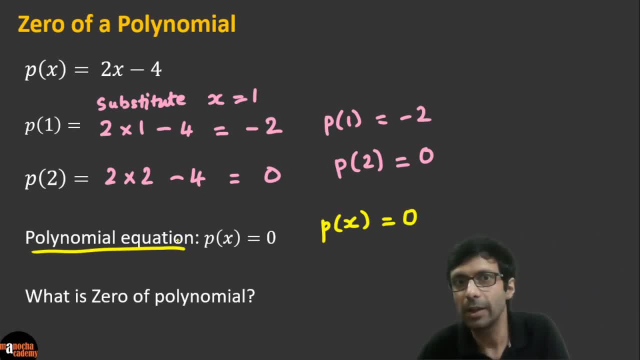 this is called the polynomial equation because the polynomial is just the expression right, 2x minus 4. but when you say it is equal to 0, an equation must have the equal to right. So we are forming a polynomial equation here. This is called the polynomial equation right. So for example, if 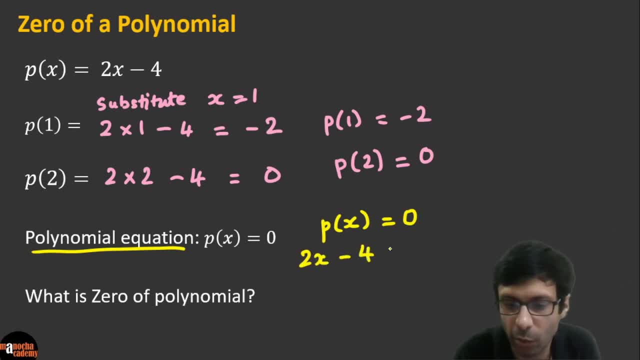 we say, if we take our example, 2x minus 4, equal to 0.. So this is our polynomial equation for our example: px equal to 2x minus 4. clear Now, based on this equation, we can say what is 0 of the. 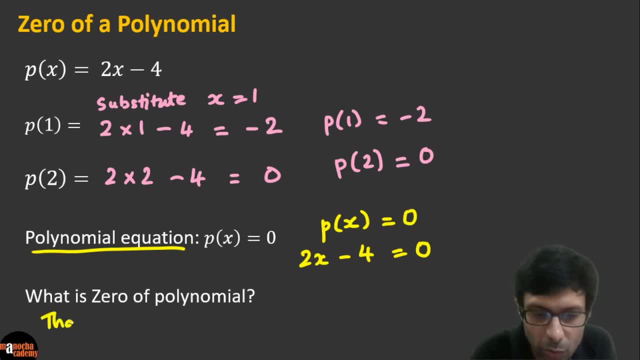 polynomial. It is that value, So that value of x, right, which makes the polynomial 0.. So that value of x, which makes the polynomial 0, okay, So guys, so basically, that value of x for which px becomes 0.. So, guys, can you tell me what is the 0 of this polynomial or example here We are talking about? 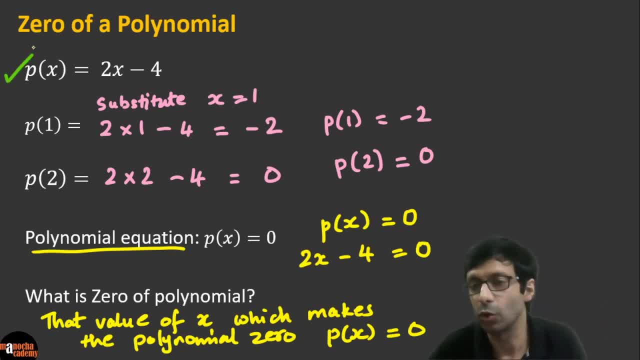 this example right on top. So what value of x? because we know we can substitute different values. what value of x makes it 0.? Excellent guys, Superb. I see Shashank Kulkarni, right, Susanta, you all have the right answer. Very good guys. So the answer is 2 because, as you can see, 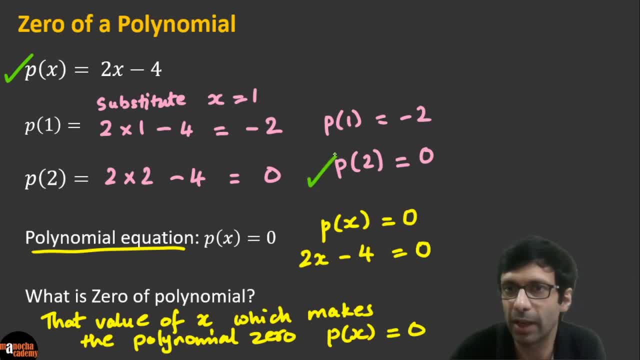 in our example here. So when we do p of 2, if we calculate for that value, the polynomial is 0. So 2 is called the. 2 is the 0 of the polynomial right, So that value which makes the polynomial zero clear. 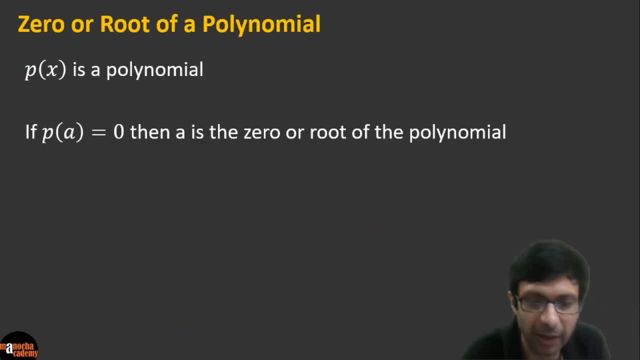 So this is called the 0 of the polynomial and we can define it clearly like this. So we can write generally that if px is a polynomial, then if p of a equal to 0. So we take any polynomial px right, and we said that p, a is equal to 0. There we have, It is the 0.. So now the other one is getting 0 point because So we Pokémon sign in and say this guy, he gets 8 points. The other one is getting opt out. So this is a fine. but So I want that far y gay, very bathroom at any rate, to forget any random stuff around this question here. So I want that, if p of a equal to zero, the 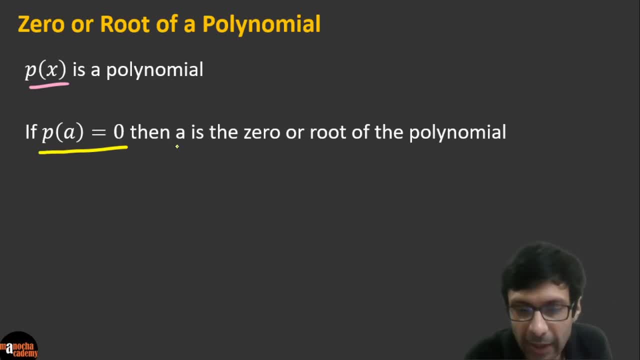 objective, Then we much better. the зов px is a polynomial right. 001 texts det powder and he says: then PA is equal to 0, then A is basically called the 0, or it's also known as the root of the polynomial or 0 root of the polynomial equation. Okay, guys, is it clear? So this is a very important. 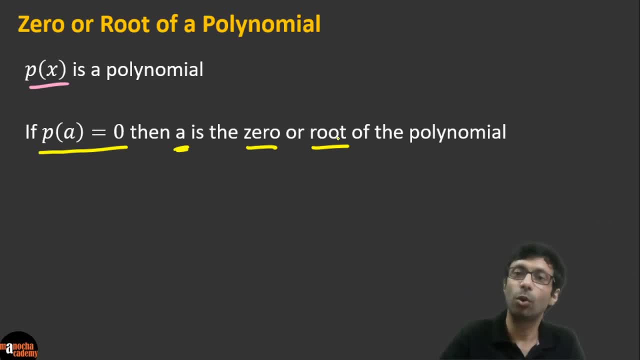 term. don't confuse this with the 0 polynomial. this is 0, or root of a polynomial, and that value of x which basically- so you can learn it like this- that value of x which makes the polynomial 0, and this is the formal way of writing it. Okay, guys, clear, Very good. 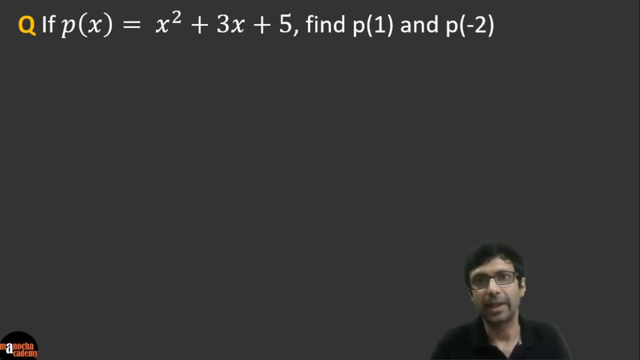 So now let's try this question. So if you are given Px equal to x square plus 3x plus 5 guys, can you quickly calculate P1 for me? So let's do the two parts: find P1 and P minus 2.. 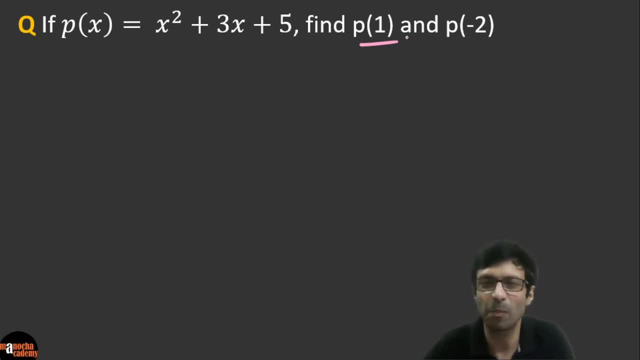 So I want all of you to try. this is a maths class, so, guys, get your pen and paper ready and go ahead and try it, or maybe, if you want to do it mentally right, you can do that. so come on. I want all of you to find P1.. So what is P1 going to be and how do we calculate it? Very simple. 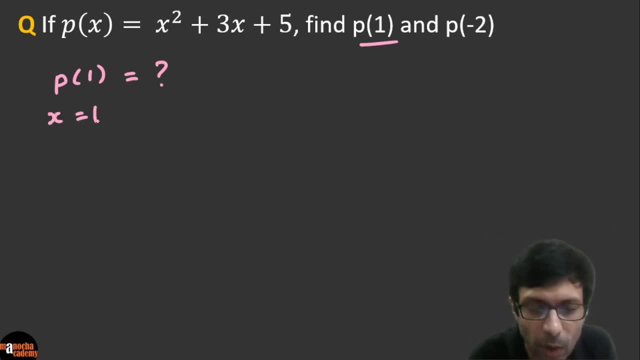 it's so easy. you just have to substitute x equal to 1 in this polynomial right? So what will P1 be? So simple, it's going to be 1 square plus 3 times 1 plus 5, right? So what is everyone getting, guys? 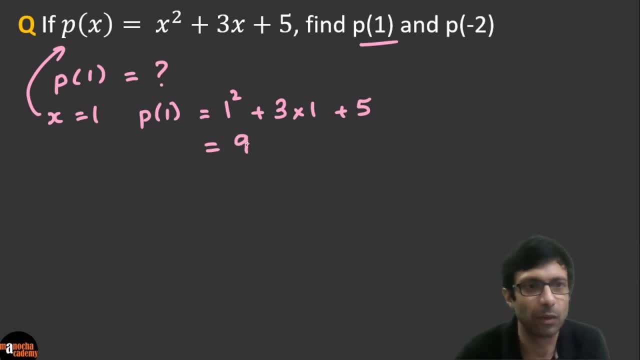 So that's basically equal to 9, right? 1 plus 3 plus 5.. Okay, excellent, clear. And similarly, guys, we can also do P of minus 2.. So we need to substitute minus 2 in the polynomial. So, guys, what are you getting for that? 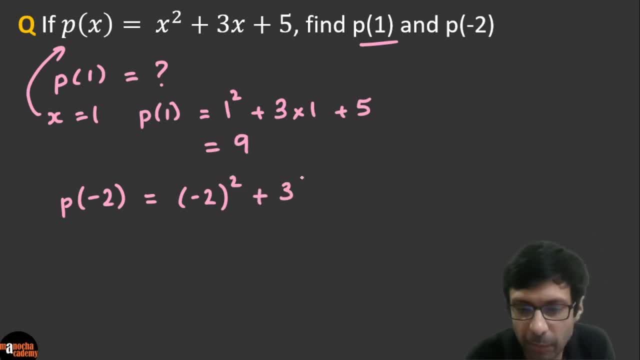 So minus 2 whole square plus 3 times minus 2 plus 5.. So what is that going to work out to? This is 4 minus 6 plus 5.. So come on, check my calculation in case I'm doing something wrong. 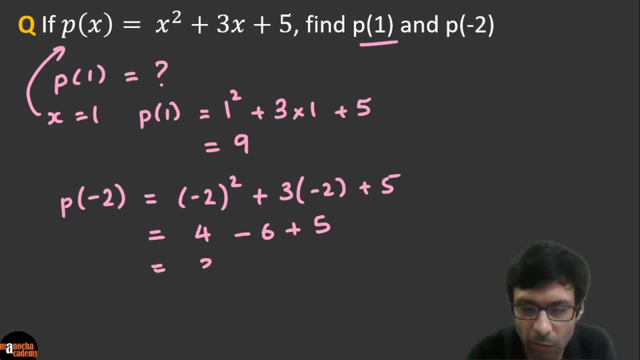 So, guys, what is the answer here? I think a lot of you got the answer 3 right, 9 minus 6.. Very good, So as simple as that. sometimes you get these really simple questions. So it's just substituting the value right, the value given in the bracket as x. Okay, very simple, right. Now I'll try this question. 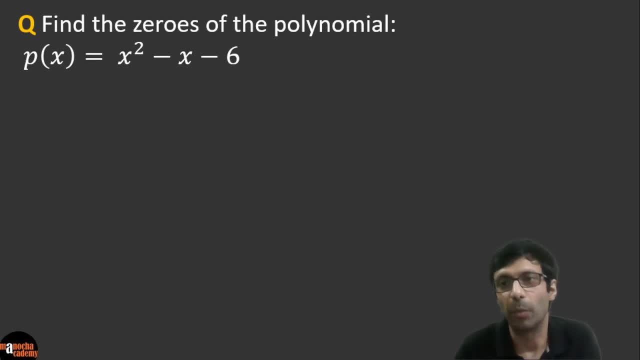 guys, Find the zeros of the polynomial. where polynomial can be, is given Px right be denoted as Px. So the polynomial given to us is x square minus x minus 6.. Okay, so, guys, can you see this is a quadratic polynomial because the degree is 2.. So find the zeros of this polynomial. Come on, I want. 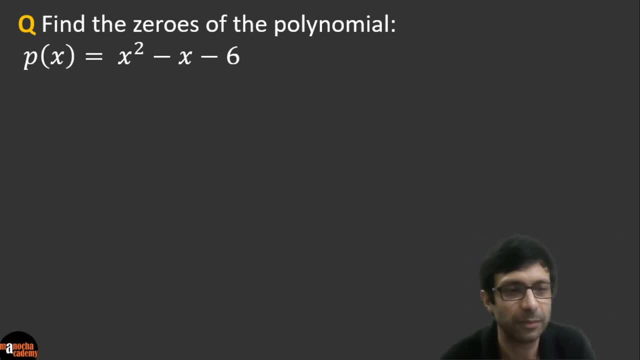 all of you to try this question Right, and what do we mean by find the zeros? guys, As we learned, it's very simple to find the zeros. you basically have to form the polynomial equation, which basically means Px equal to 0, right? So we set the polynomial equal to 0. So that's our equation. 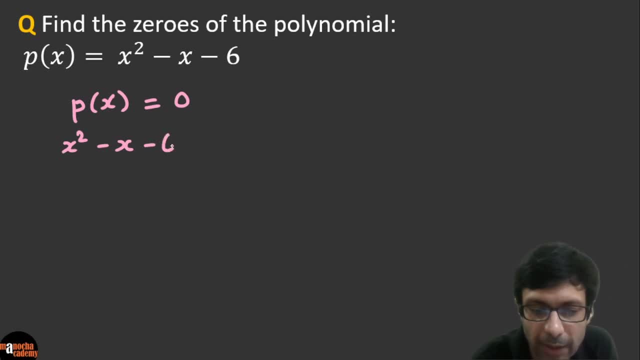 So we say x square minus x minus 6, equal to 0.. And so to find the zeros of the polynomial, basically you need to solve the equation for x, right? So what is the meaning of zeros of the polynomial? You solve the equation right here. So to find it, you need to solve for the values of x. 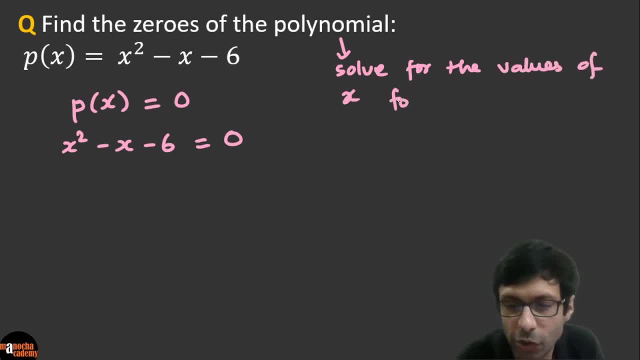 right, For which Px is 0. Clear, So this is how you find the zeros of the polynomial. So, guys, come on, solve that equation. It should be pretty simple, right? So for what values are you getting this? Okay? very good, I'm seeing some right answers there. So how do we solve this, guys? 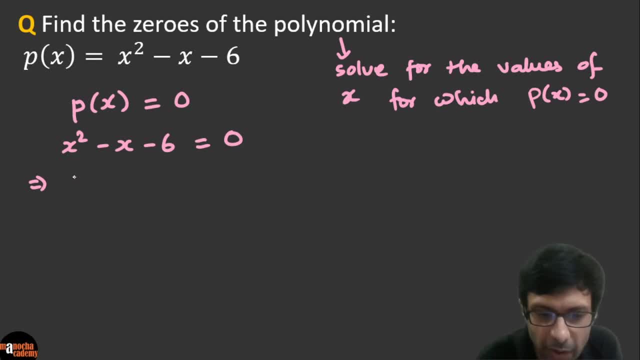 So we basically need to factorize this equation, right? So what are the factors going to be? So the first one is x minus 3, right? So, guys, can you see what are we doing To find the zeros? we are basically factorizing it to solve it, right? So now you can see. so either x plus 2 can be 0 or x minus 3 can. 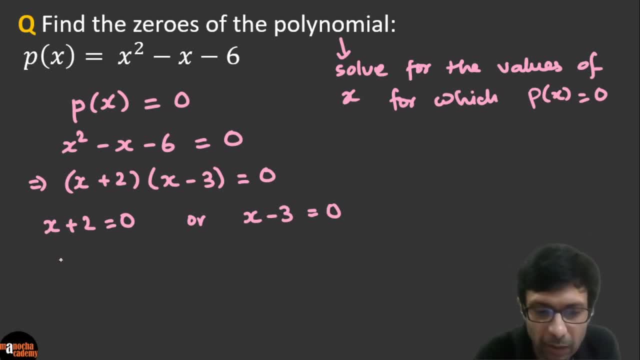 be 0, right, Simple. So what do we get here? x equal to minus 2 or x equal to 3.. Okay, guys, So check my answer. Did I do some mistake, right? Is my answer correct, guys? So what have we found? 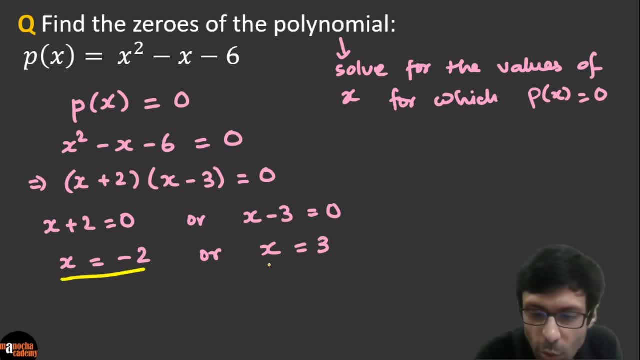 So these are the values. So these are called the zeros of the polynomial. So the zeros of our polynomial are basically going to be minus 2 comma 3.. Those values of x for which the polynomial becomes 0. Okay and guys, if you're having a doubt, just follow me. Very simple, So we've been given. 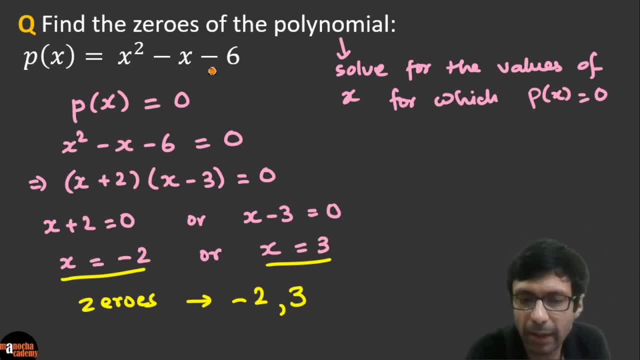 some of you are having a doubt. So, all right, I'm repeating: x square minus x minus 6.. This is our polynomial. Our goal is what? Always look at the goal, right, Just like what's the goal of in your life, right? So you should always work with the goal in mind. So what is our goal? We need to find. 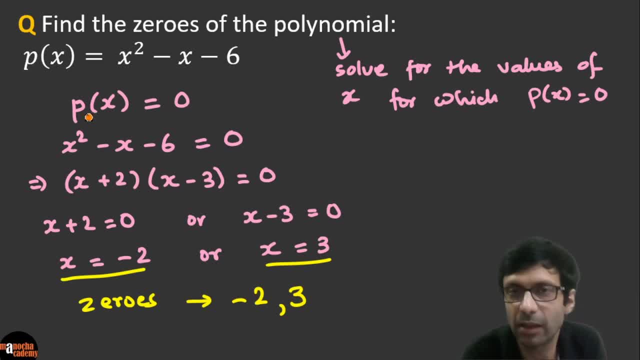 the zeros. So basically, we take the polynomial and set it equal to 0. That's what we want and we need to solve. So we've got this equation: x square minus x minus 6, equal to 0. Now, basically, equation. So that will give us the values of x, for which it's 0. right, The polynomial is 0, and how? 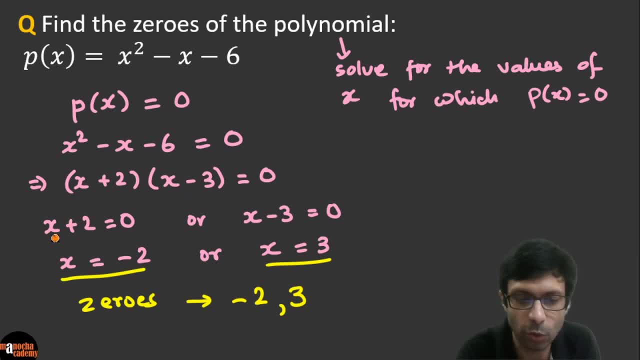 do you solve it? You just factorize it right and you do that. So what do you get? x plus 2 equal to 0, or x minus 3 equal to 0, and then basically you get these values Clear. So we get x equal to minus. 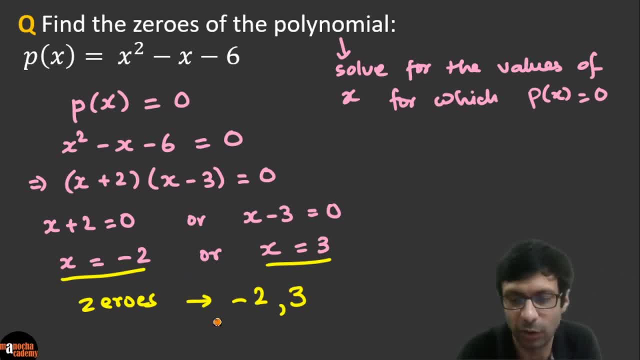 2 or x equal to 3, and those are basically our zeros of the polynomial, Very simple. So once you get it, it's really easy, right, And guys? if you have any doubts, you can put it in the comments below or go back and watch the replay of this class and I think you'll get these concepts pretty clear. 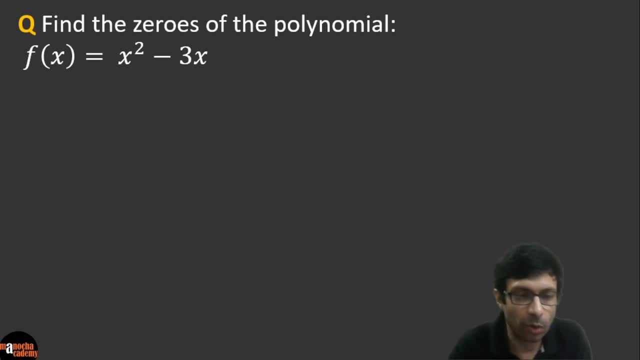 Now find the zeros of this polynomial, right? So remember last time it was called px, This time it's called fx, right, You can use any notation: px, fx. you can even have gx, right? Whatever letter you want to use doesn't matter, right? So it's a polynomial in the variable. 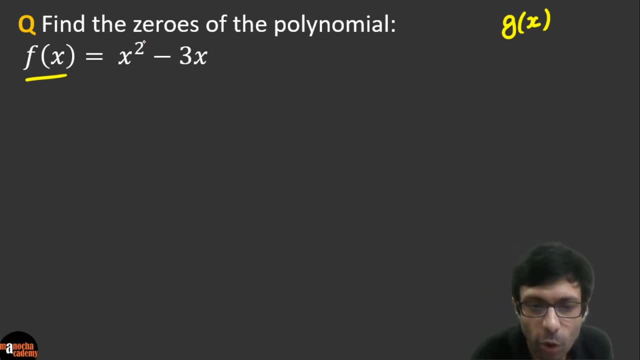 x and we need to find its zeros. So, come on, I want everybody to try this. Use the concept we learned Very good, Some of you already writing the answers. Wow, you guys are really fast, Okay. so how do we do this? guys Remember to find the zeros. basically, we need to set the polynomial to 0 because we want 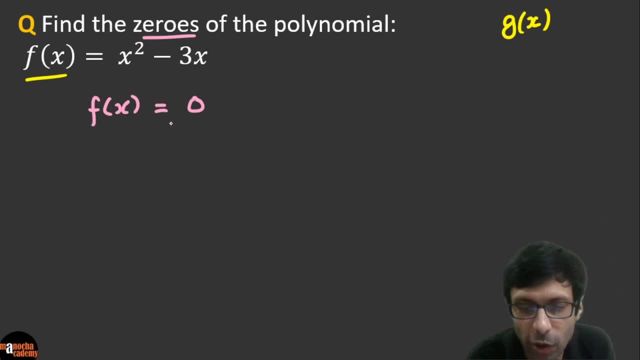 to find the values for which the polynomial becomes 0.. So this is our equation: x square equal to 0.. This is the important thing, right? This is our equation. Please take a look. So very simple to get the equation, just put it equal to 0. Clear. Now you need to solve for the values of x. 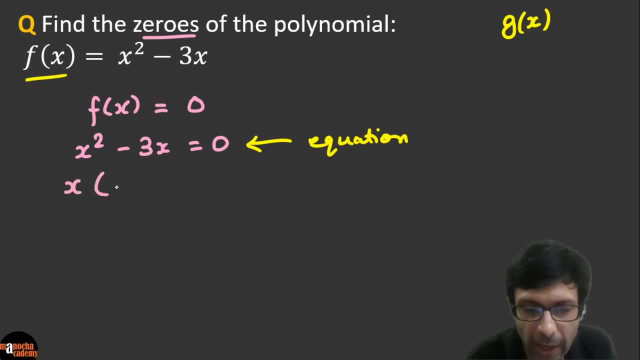 So how do we do that? So again, we'll factorize this. So it's going to be x times x minus 3 is equal to 0.. Okay, right, And so this polynomial. guys, what degree was this polynomial? Okay, See, it was a quadratic polynomial, because it's a degree 2. right, x square is there and we are. 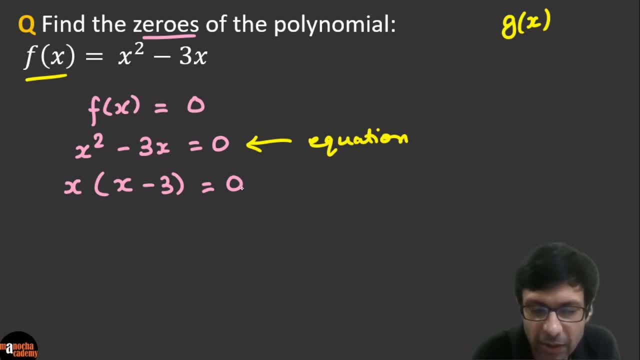 solving this. So we can say: either x is equal to 0 or x minus 3, right? So either x is 0 or x minus 3 is equal to 0.. Okay, because either this term can be 0 or this term, right guys? And so so either x is, 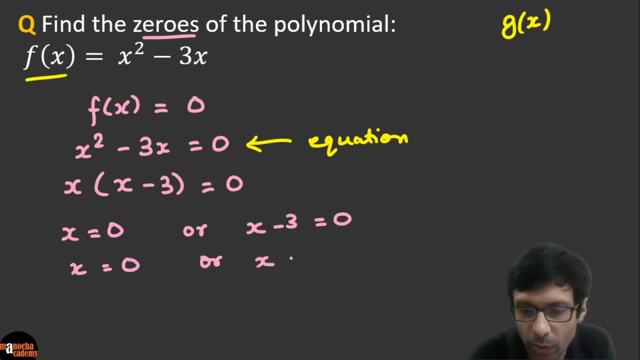 0 or x is equal to 3.. We take the minus 3 on that sign. So what are our zeros of the polynomial? The values 0 and 3.. Excellent, I see a lot of you got the right answer. So zeros of this polynomial. 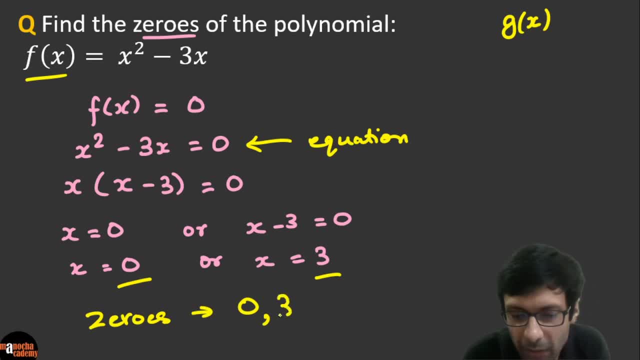 becomes 0 comma 3.. Clear, Okay, And you can go and double check it also, right, You? if you want to check your answer, what do you need to do? A very simple way to check the answer: You take f of 0.. So let's find f of 0. 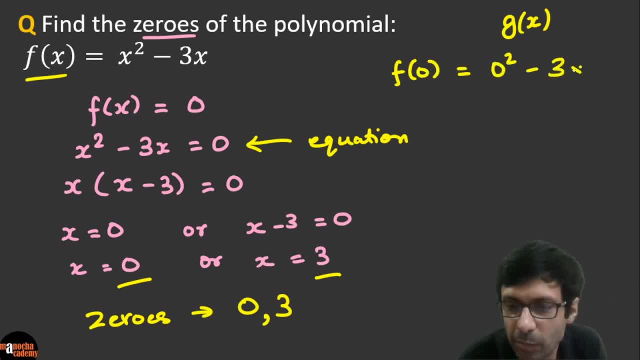 So that's going to be 0 squared minus 3 times 0. See, we are getting 0. And take again f of 3.. So go back and substitute it. So f of 3 we've taken, So that's going to be 3 squared minus 3. 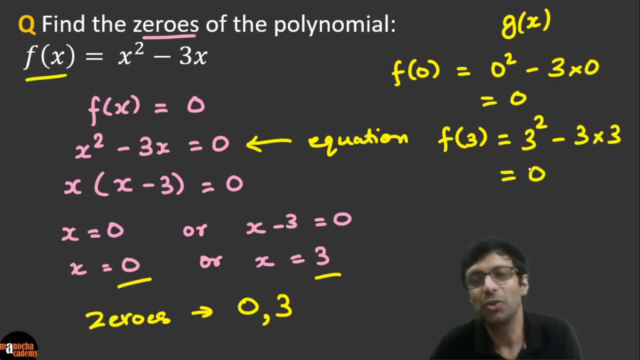 times 3.. So 9 minus 9, again 0.. So see, guys, you can quickly confirm your answer, right? So whatever values you've got, go ahead and substitute it in the polynomial and basically you should get 0, because your goal was to find the zeros of the polynomial. 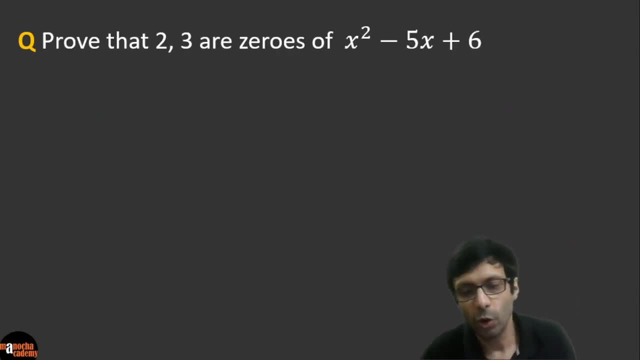 Okay, Now go ahead and try this question: How do you prove that 2 comma 3 are the zeros of this polynomial? All right, guys, everyone, I want you to try this question And you guys have been superb, really interactive, and you're answering so many questions right, So it's great. 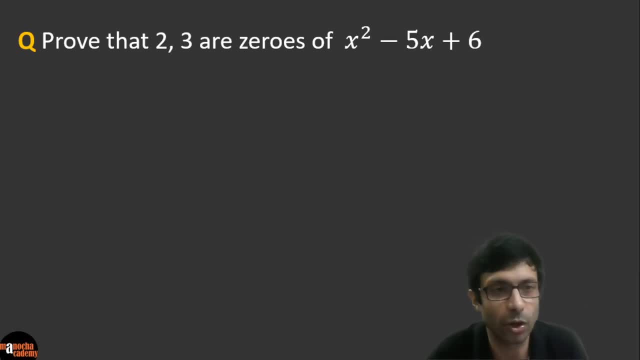 to see that in the chat. guys. I really find that awesome that everyone's participating in these sessions. So go ahead and try this question and if you haven't hit the like button, please hit it right now And share it out with your friends so that we can have more folks on these sessions. Okay, So how? 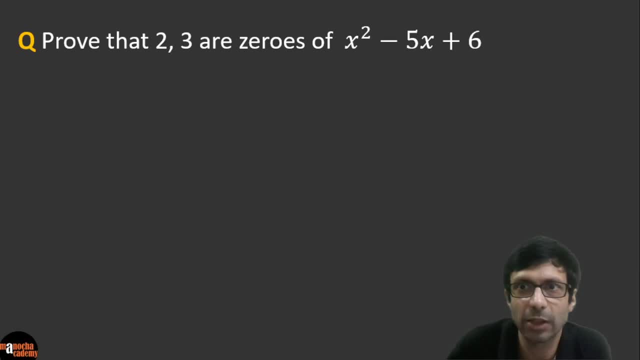 do you prove that 2 comma 3 are zeros of x squared minus 5x plus 6.. So somebody's saying by factorization, Somebody's saying by verification: Okay, So how do we find this right? Okay, So actually you don't need to factorize here. This question is pretty simple, So we'll just do I. 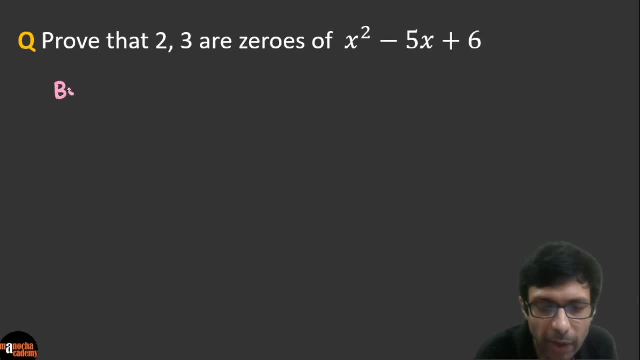 think someone said that correctly. I missed the name. So by verification, Okay, So how do we find this right? Okay, So, actually, you don't need to factorize here. This question is pretty simple. So by verification, right, Right. So what do we mean by verification? To prove that these are the 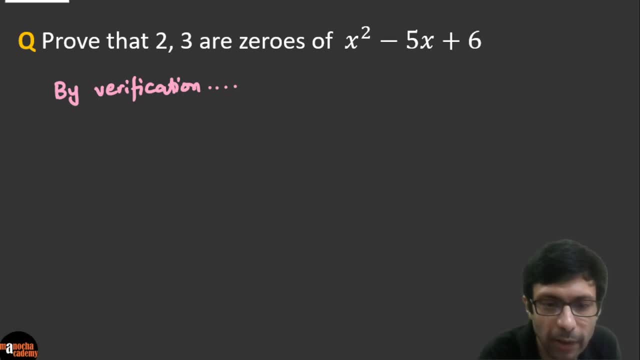 zeros of this thing. So first let's write the polynomial clearly. So our polynomial fx is basically: So: always write it clearly: fx equal to x squared minus 5x plus 6.. That's our polynomial right, And we need to prove that 2 comma 3 are zeros of it. So what is the verification Basically? 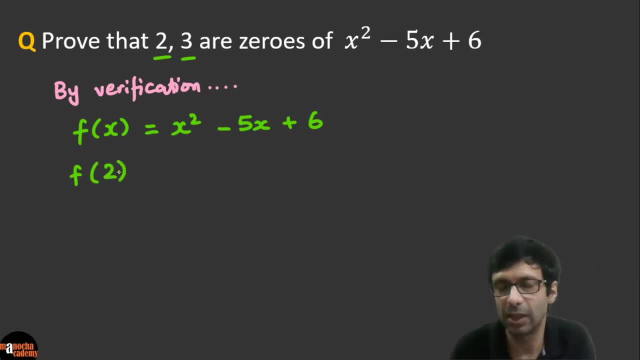 we need to find. Let's say, 2 is a zero of the polynomial. Then we find f of 2 and that should turn out to be zero, Right? So let's check that. So what is f of 2.. 2 squared minus 5 times 2 plus? 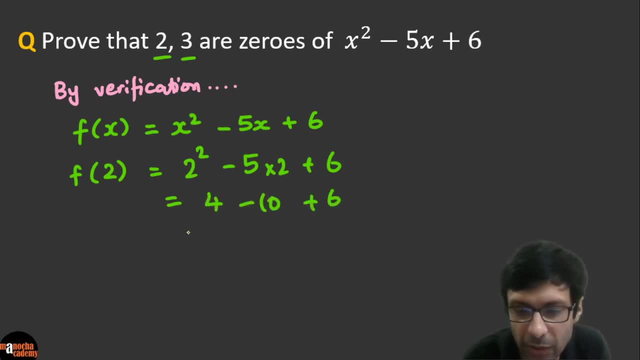 6. So that's going to be 4 minus 10 plus 6.. Right, And guys, you can see it's zero. So we have verified, since f of 2 is zero. Therefore, absolutely right, 2 is a zero of the polynomial. 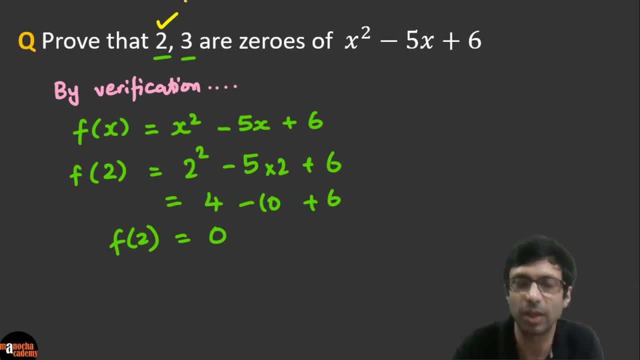 Score back. verification. You don't have to factorize that, You just need to substitute it, Right? Just like in the previous question, We were verifying our roots. You saw that we did that, So the same technique here, Right? Similarly, guys, you can try it for the f of 3, right? So to verify that. 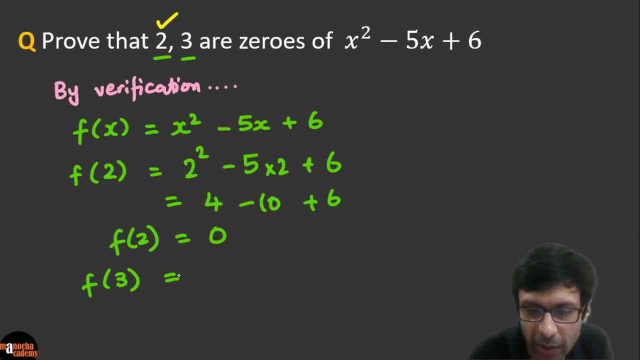 3 is a zero or a root of the polynomial, We find f of 3.. So that's going to be 3 squared minus 5. that's going to be 9 minus 15 plus 6.. And, guys, again we get 0.. Okay, So f of 3.. Very good A lot. 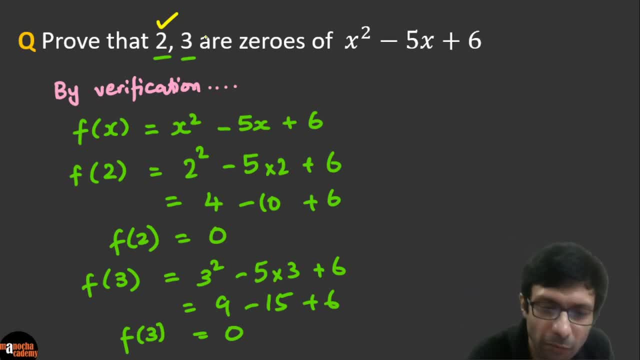 of you are doing that, You're calculating. So this is a very simple question, Very easy to verify, Right. It's like almost a giveaway thing that you just substitute and check it Right And you can see we've clearly verified the. these are the zeros of the polynomial. All right, Excellent guys. 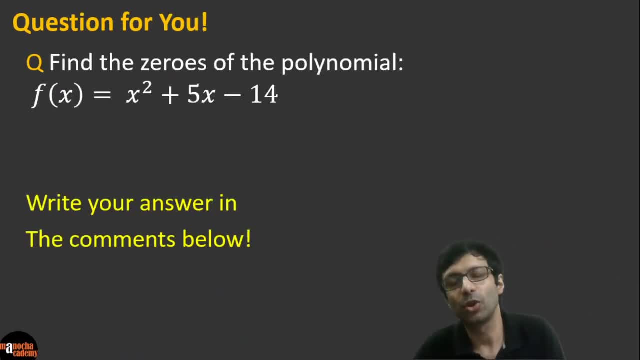 And now I have an interesting question for you. Find the zeros of the polynomial fx equal to x squared plus 5x minus 14.. Okay, And this is your homework question. So I want you to write the answer in the comments below And I promise to reply to. 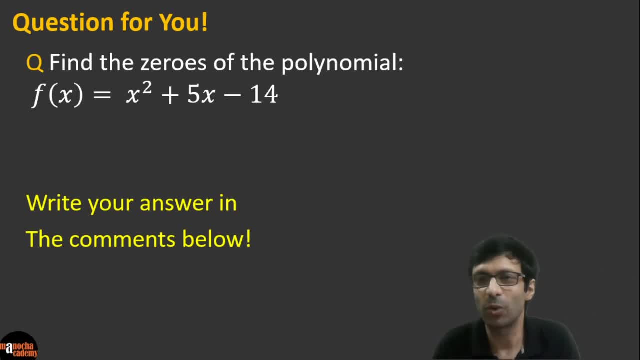 your answers as soon as possible. So, guys, we won't discuss this question because I want everyone to revise the polynomial chapter, Be clear about all the different terms we've learned. We talked about zeros, right of the polynomial, And do write your answer in the comments below, Right And. 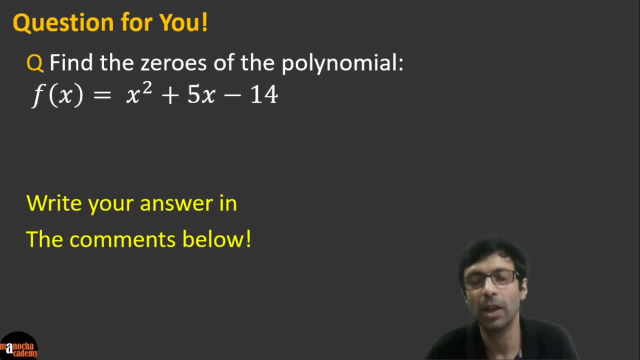 in a future class we'll talk about the remainder theorem, the factor theorem, So I won't go into that in this class. So, guys, go ahead and try this question and do write your answer in the comments below. I look forward to reading your comments. And, guys, as I said, we've got this website. 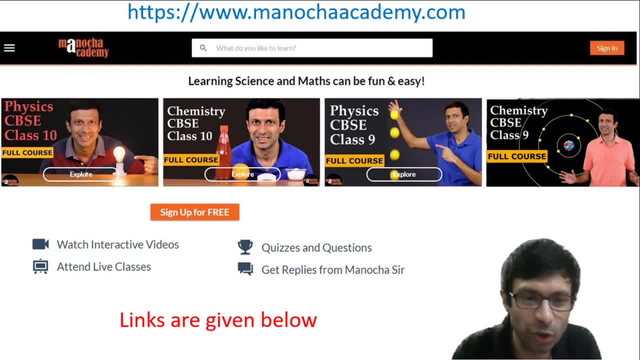 manochacademycom. So do check it out. And just today we launched this new course, Right The chemistry CBSE class 9 course. So, guys, those of you who are interested, you can check it out. These courses are very useful for you, for your preparation, And we have big discounts going on. 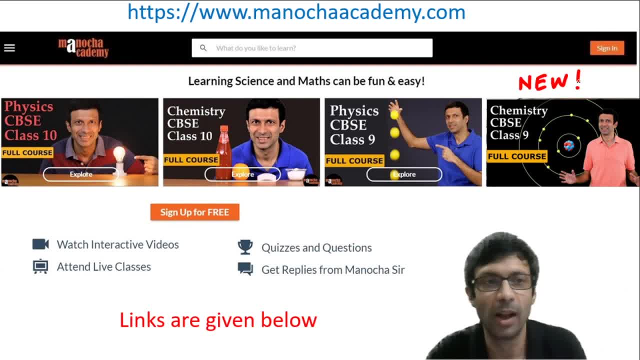 So do take a look. I think you'll really find them really helpful And they have interactive videos. We're going to be starting special live classes also in these courses and quizzes and questions, So it's really useful And I'll put the links below. And, guys, if you haven't subscribed to our 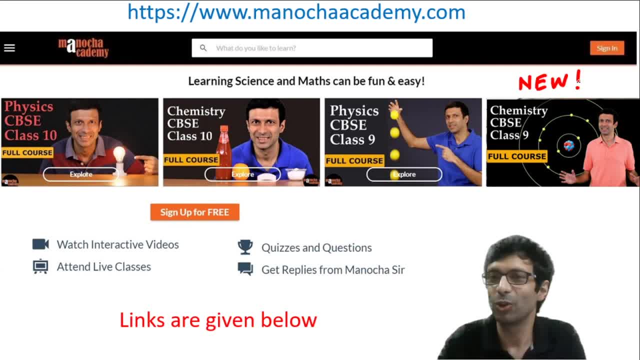 YouTube channel. please hit the subscribe button right now and click on the notification bell so that you don't miss out on these live classes That we are having at 8 pm daily on physics, chemistry and math topics. And guys, you can give your feedback on what topics you would like in the live class. So I may not be able to take. 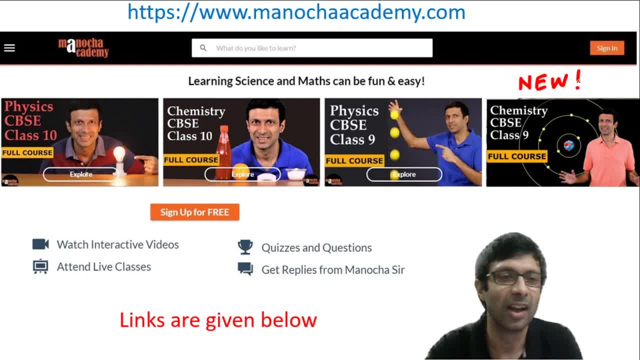 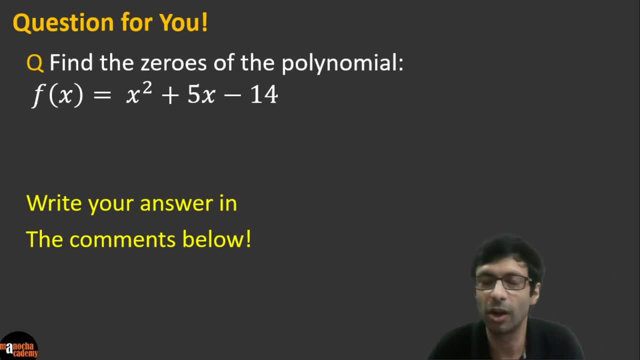 each one of them. but we can go for you know majority votes and see which one is the having the largest voting Right, So do put in the feedback in the comments and try this question. And, guys, it's really amazing to read everyone's comments and feedback. I really enjoy reading. 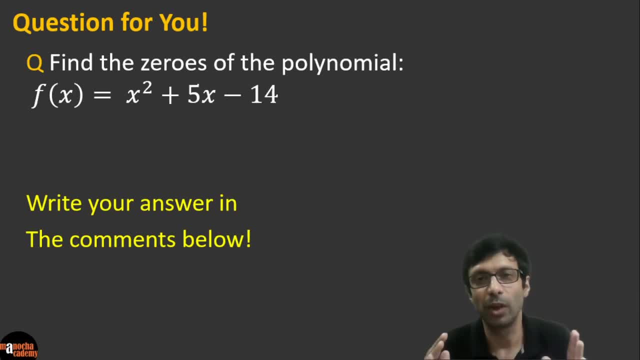 them, and a big thanks from the Mnuchin Academy team. We're trying to bring you awesome content on physics, chemistry and maths, So I hope you enjoy our videos and classes, And thanks a lot, guys, for joining into this maths class. It was wonderful seeing everyone's participation, So 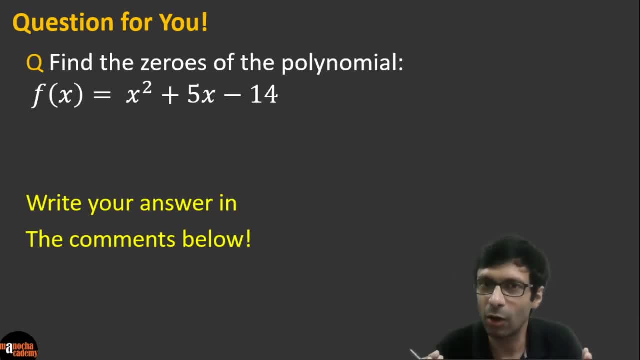 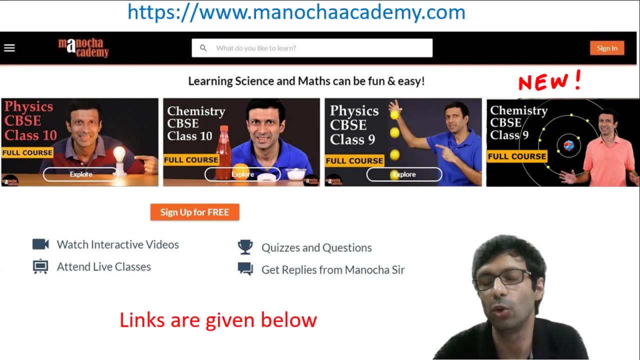 guys keep practicing, Keep working and take care of your health, also during this lockdown period. So I pray for everyone's good health and, guys take care and keep your studies and preparations going. to help you with that, We've got our website, mnuchinacademycom, and you'll really find these. 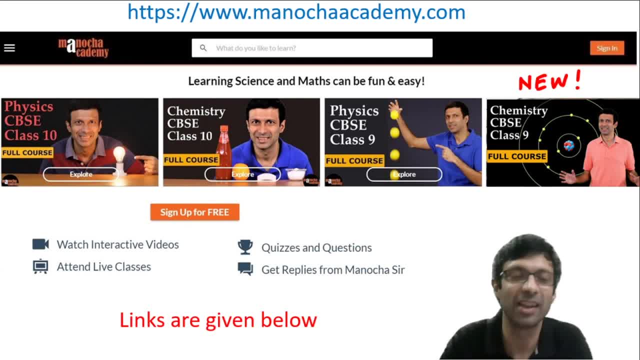 courses very useful, So do take a look and guys share it with your friends. Thanks a lot. I really enjoyed the class and hope you did too. All right, guys, take care bye, bye And do join us in the next live session as well. I'm hoping to see all of you there and all of your friends as well. All right, bye, guys.